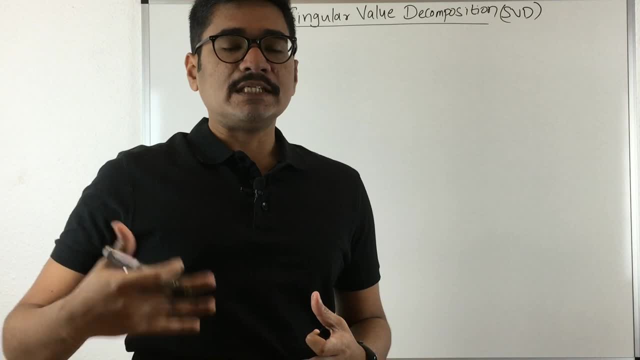 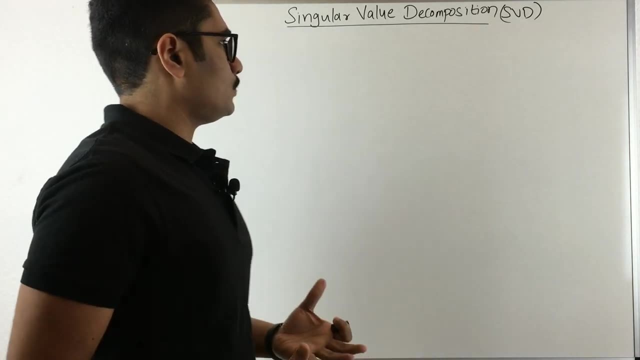 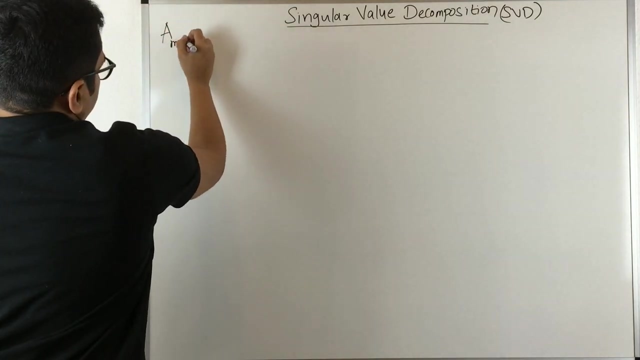 but here we have a different scenario, that is, we consider different types of matrices, So the basic definition, or when we do the decoding of singular value decomposition, we get the idea that whenever you have a matrix, say a is a matrix of size m, cross n, it will. 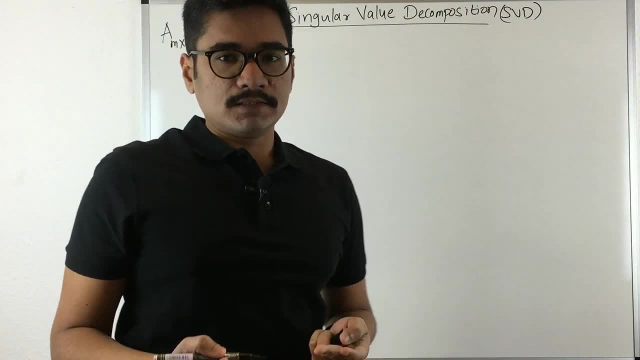 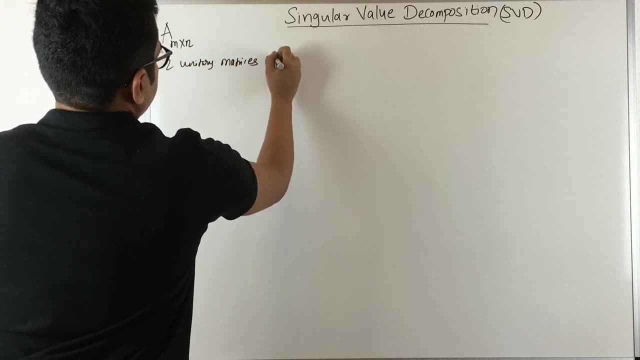 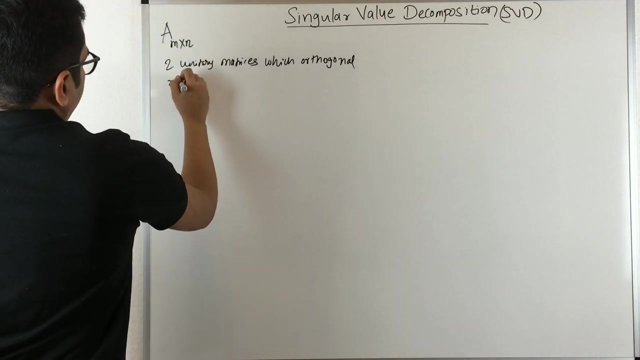 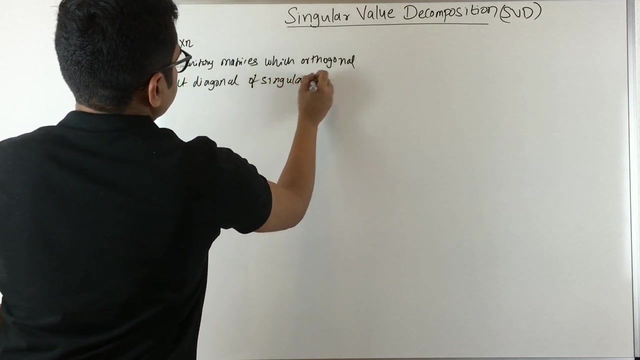 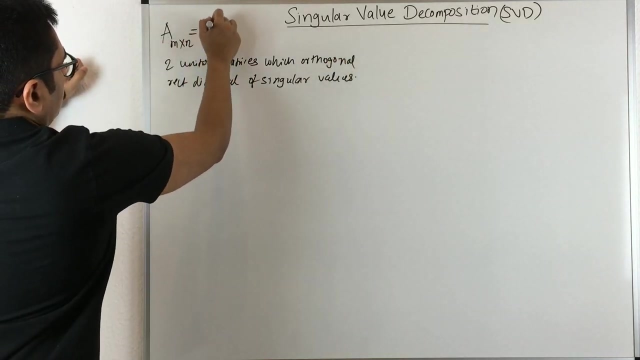 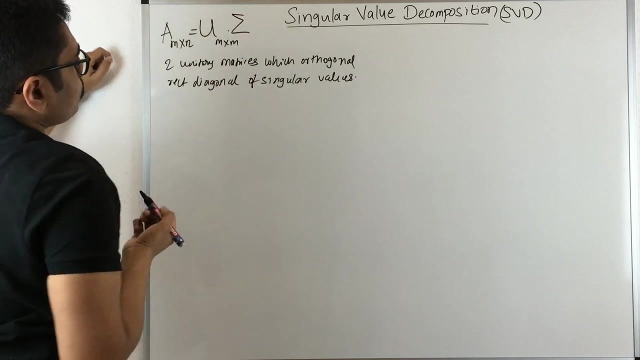 divide this matrix into two unitary matrices: Two unitary matrices which are orthogonal in nature And a rectangular, diagonal matrix of single, singular values. So when we write in the basic terms, you have a matrix, U, which is of size m cross m. then you have a singular value matrix which is diagonal in nature, that is, m cross. 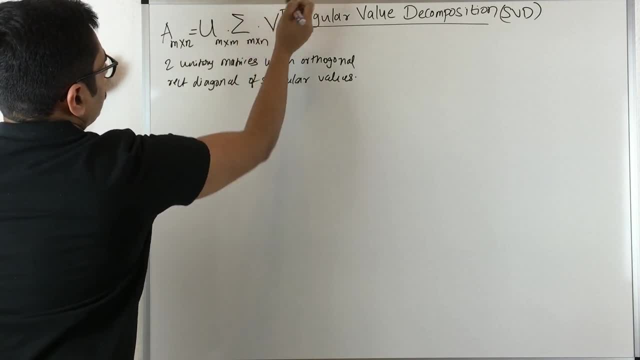 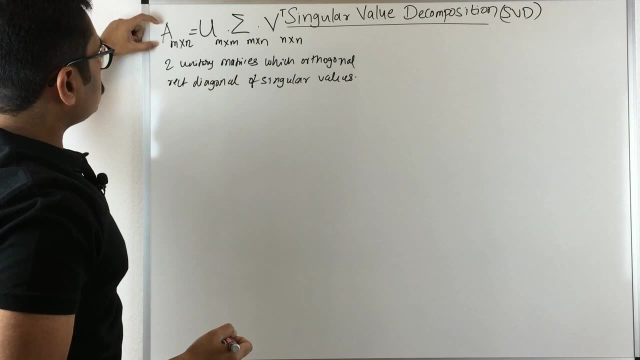 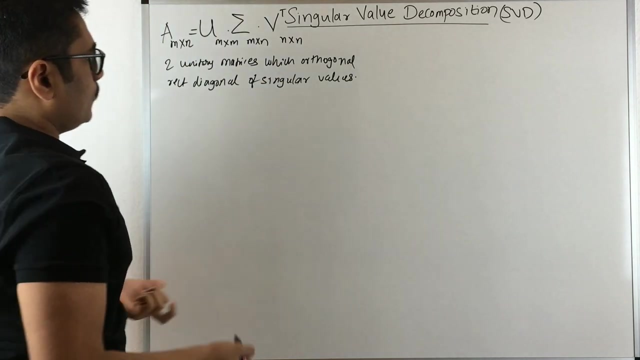 n and then you have a V transpose which is n cross n. So this is the basic three elements of how we decompose any matrix into three of this component. So this is basically what we achieve in singular value decomposition. Now there is one property of this orthogonal: 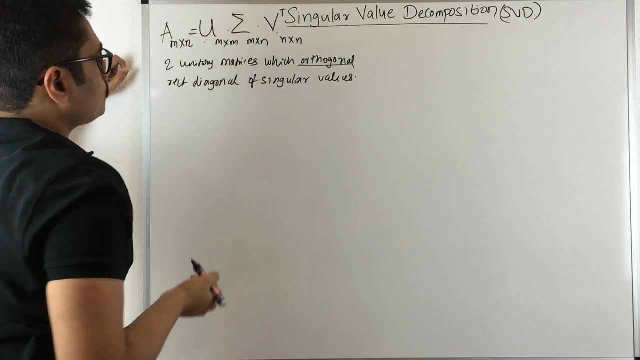 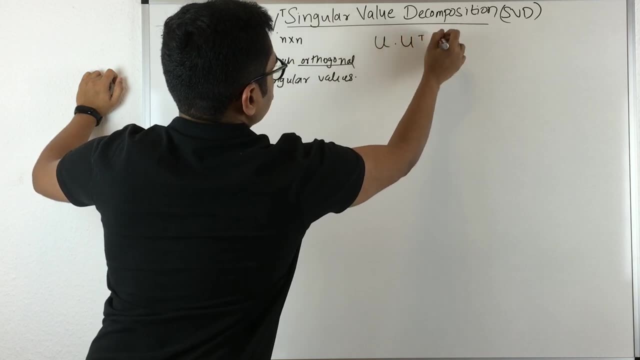 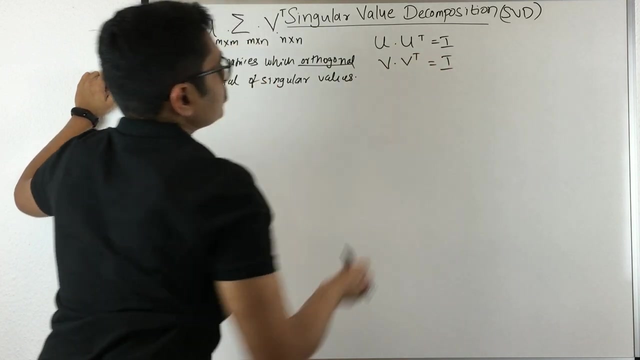 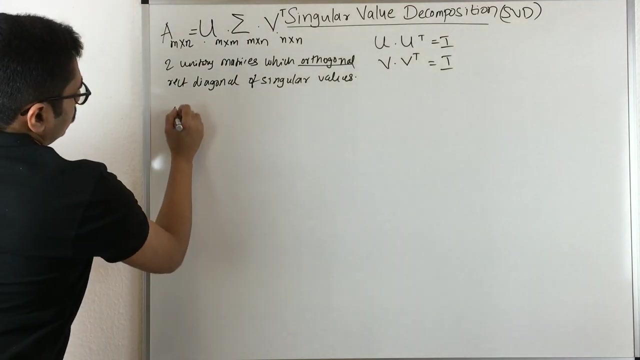 matrixes. So this is orthogonal and this V transpose is also orthogonal. Now you have this U, so you take U and U transpose, which becomes identity matrix, and similarly for V and V transpose, It becomes an identity matrix. Now, given this matrix a, what we'll do is we take the transpose. 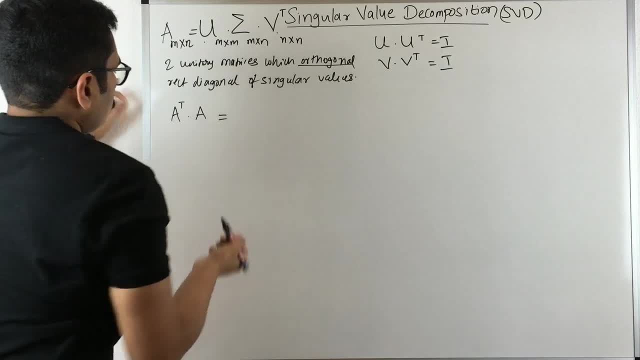 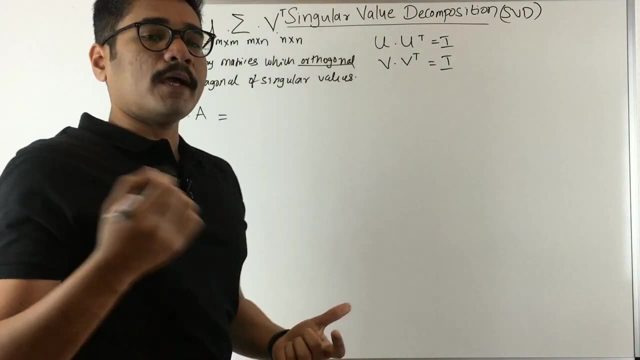 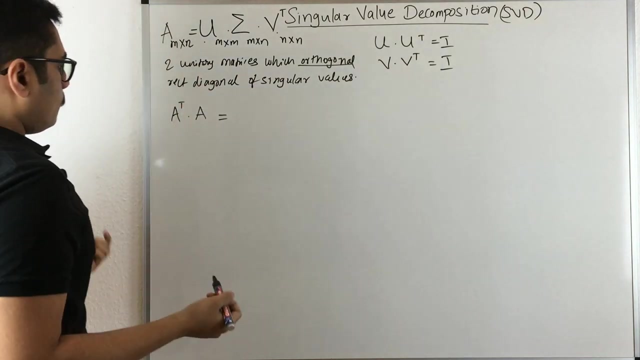 and we just multiply with this a. so what do we get? these are basic identities that will be using throughout this. So when we solve certain problems, will be coming up across different types of matrices. So just for a basic understanding what is actually happening, will do some kind of operations over this. 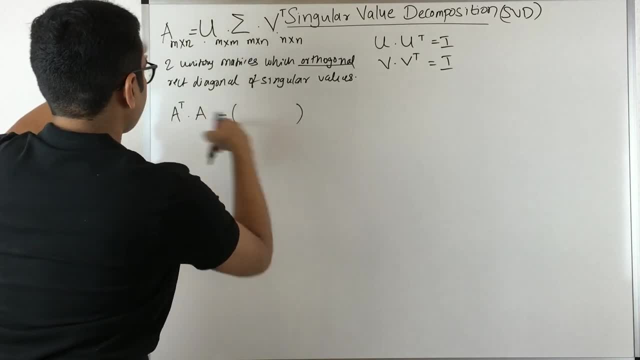 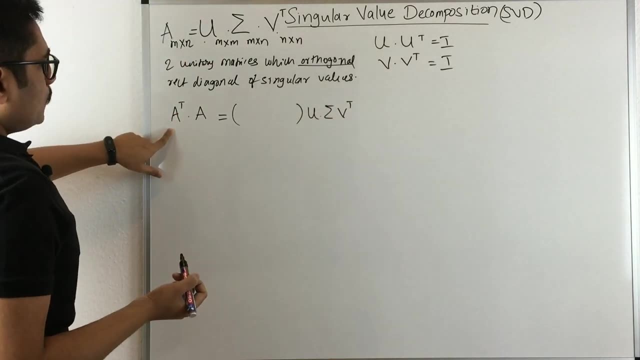 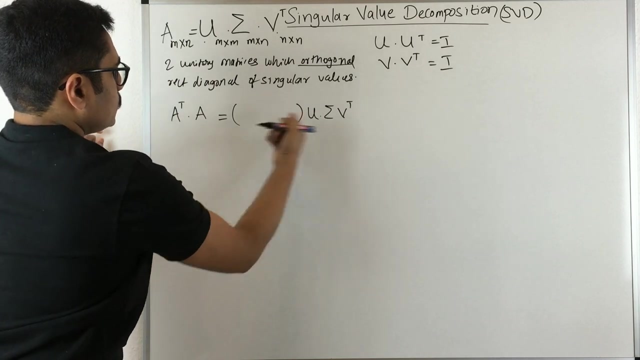 So So we have to write the transpose, and we'll just write the a matrix over here, that is U, Sigma and V transpose. now, whenever you do the transpose, what happens is the rows becomes columns or the columns becomes a rose. So you just have to reverse this. So what happens? 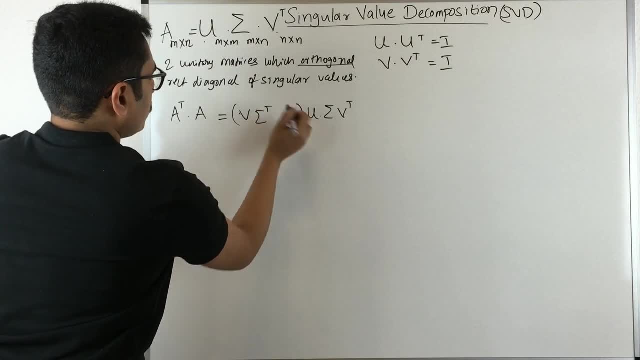 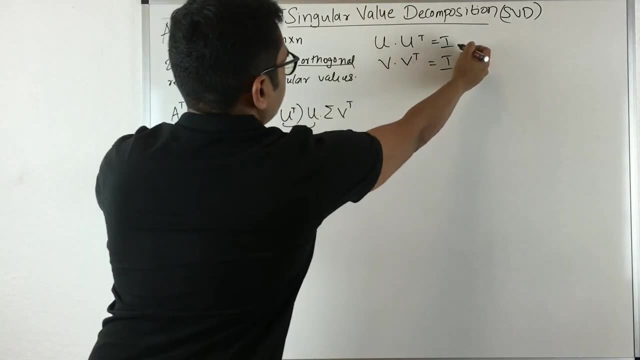 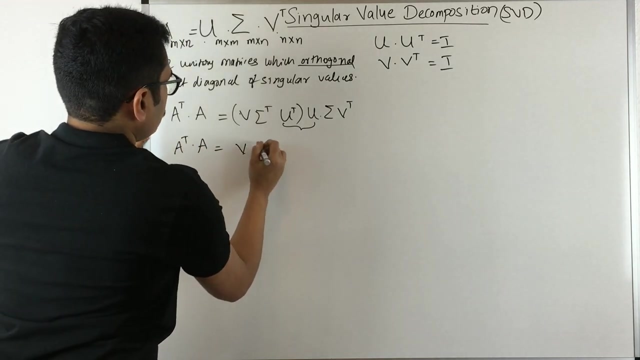 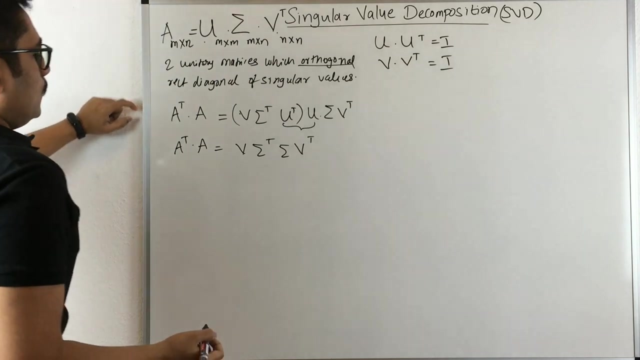 is you have V, then Sigma transpose and U transpose. now, if you just look into this term, with this identity it will be: I leaves an Opt matrix. So what do you get as an end result? a transpose is we. then you have sigma transpose, Sigma and V transpose. so this particular V matrix that is at the 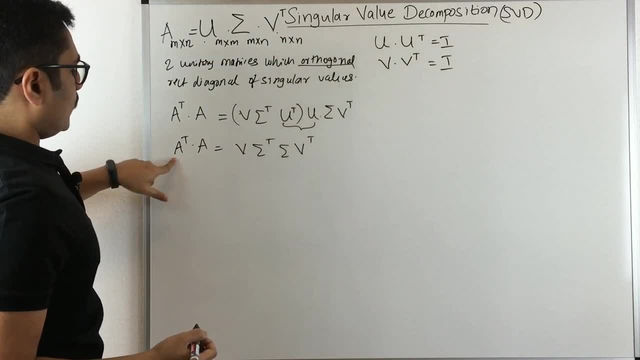 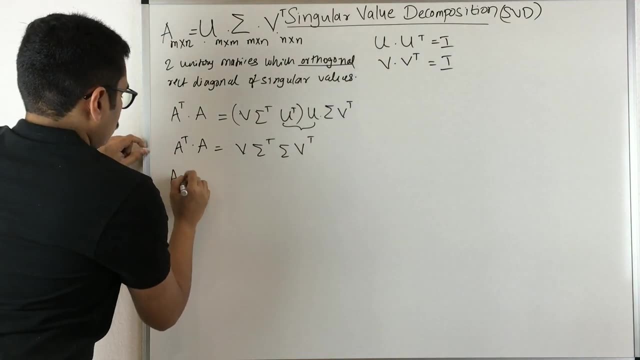 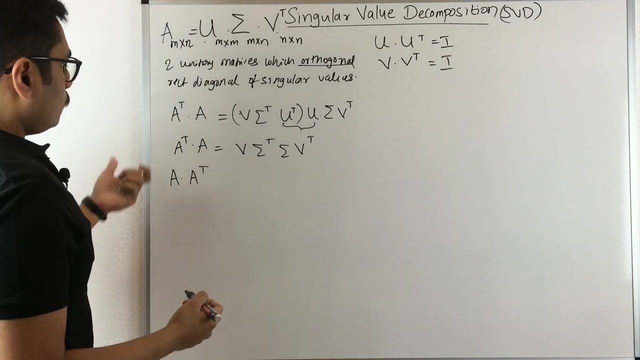 right side is obtained with the help of this operation. that kerわ this: whenever you take a faithless, you get theZeng Now-on-the-other-hand in the general Ouais. what if we do a and a transpose? So this is two different things. So we need to remind. 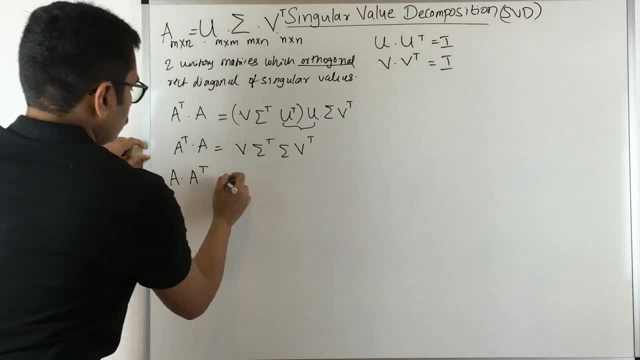 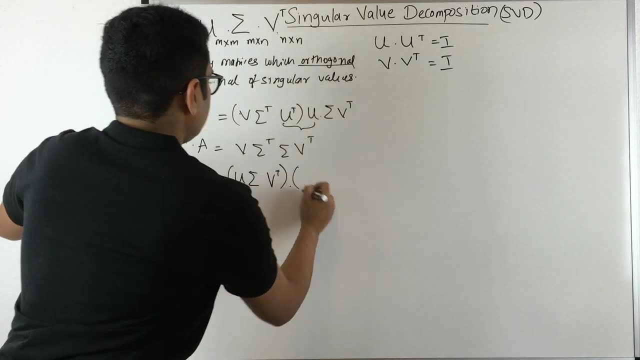 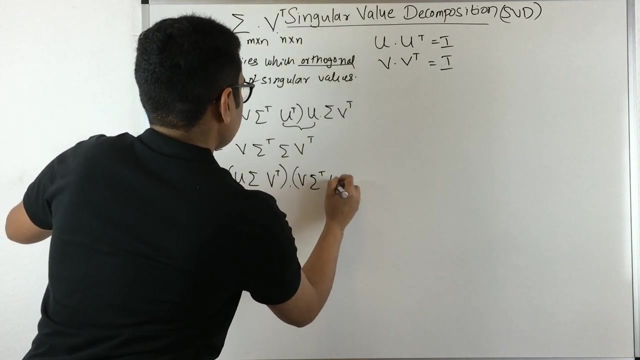 that the order of matrix multiplication is different. So with the similar notion, you go with u Sigma and V transpose, and then you have to reverse this, that is, you have V- Sigma transpose and u transpose. Now, if you look at this with this equation, it's an identity. 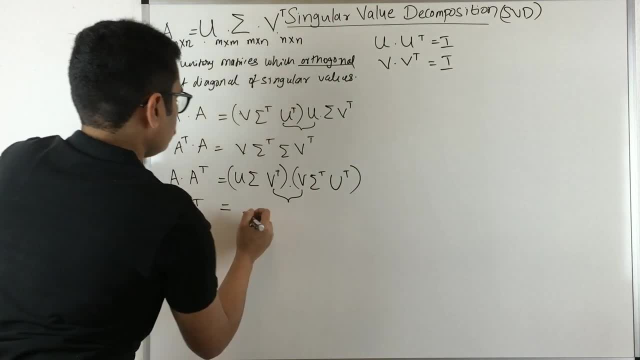 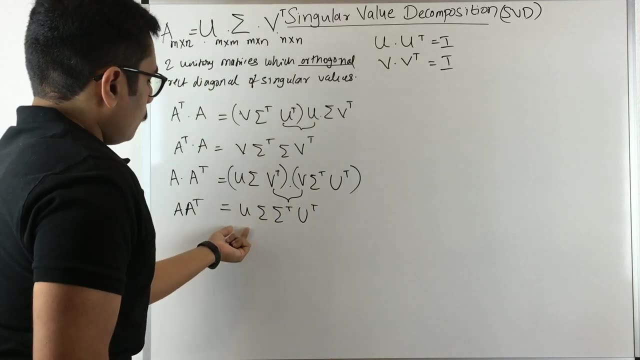 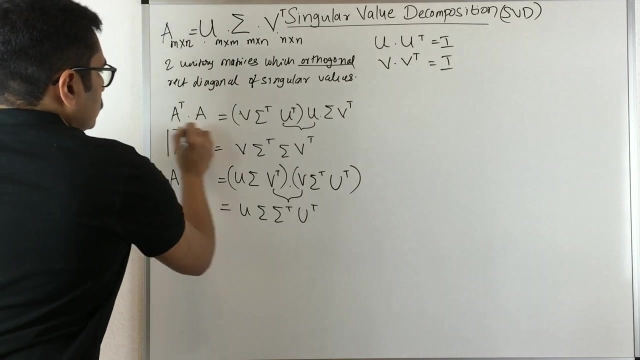 matrix. So what you have is a, a transpose becomes u Sigma, Sigma transpose and u transpose. So for obtaining this orthogonal matrix, you have to perform this kind of operations. Now, we did these many things, So what is basically happening over this? 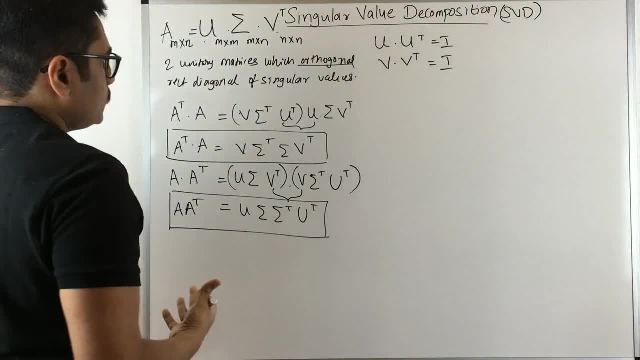 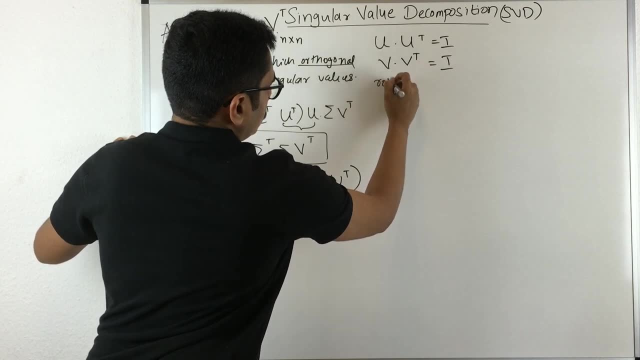 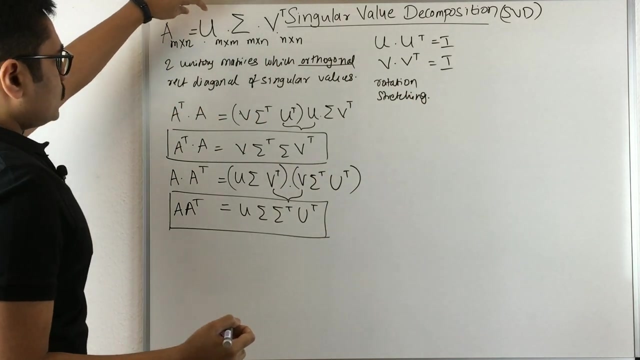 So, So, whenever in SVD, wherever we have matrixes, so we have to remind that there are two operations or two geometrical operations that is being performed, that is, rotation and stretching. So essentially, from this matrix is what we can obtain is this: u is nothing, but we just 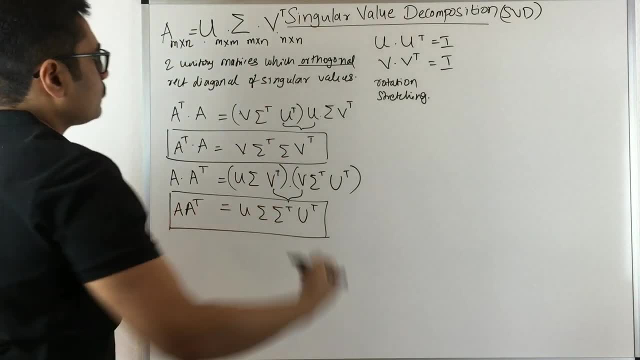 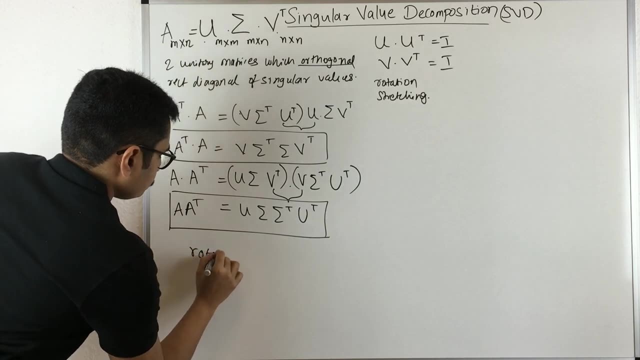 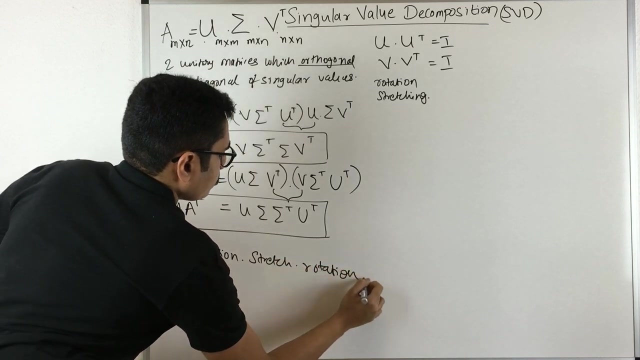 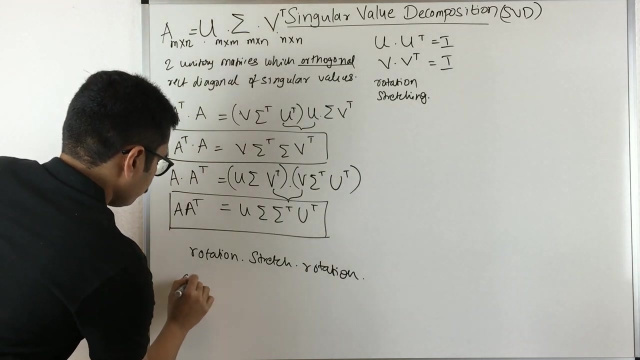 rotate that Matrix. Sigma is we stretch and V transpose is again what we do is a rotation. So it's basically rotation, stretch and rotation. So how do we rotate some particular Matrix? say we have this: cos theta minus sine theta and sine theta and cos theta. So this is basically 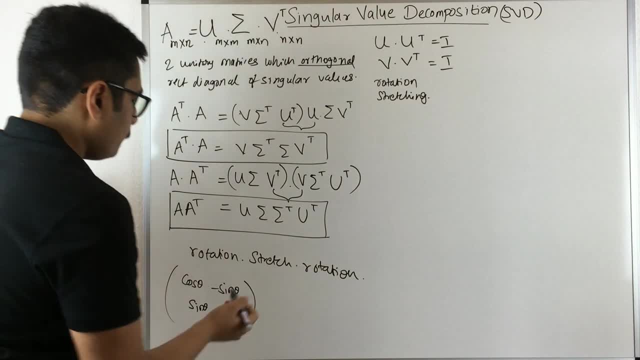 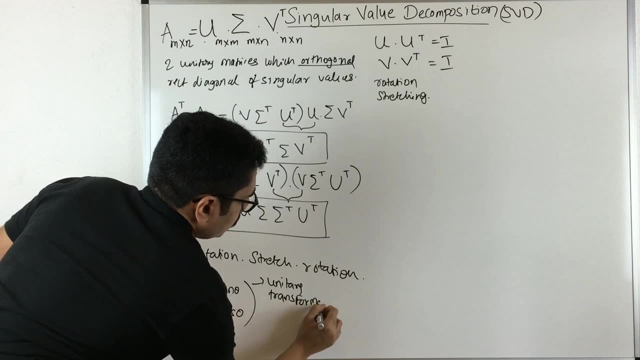 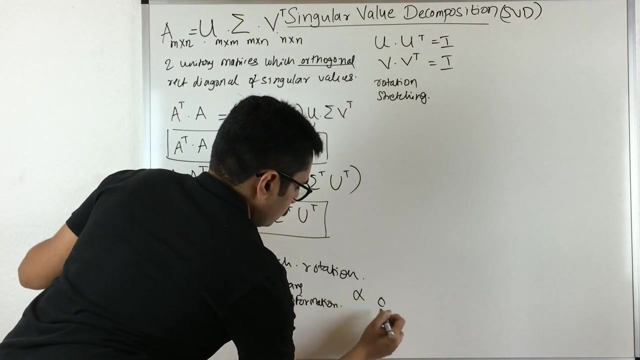 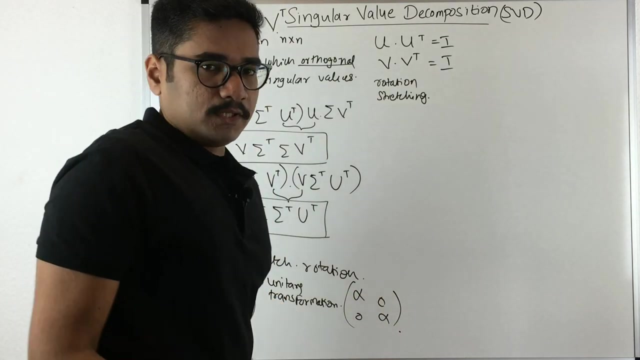 the rotation Matrix, but essentially in SVD we call this as unitary transformation. So why? because we are performing this operations over to unitary matrices and then for scaling, what we have is: we scale with some parameter, say alpha. now what is happening graphically? 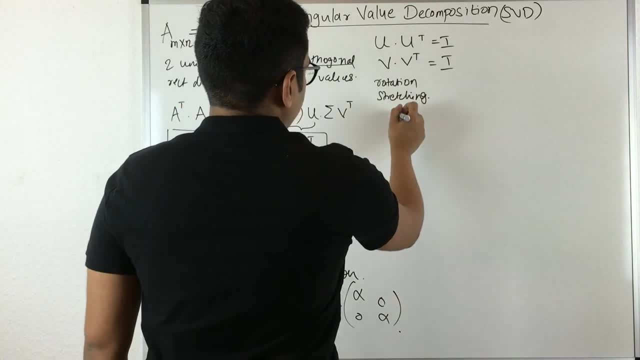 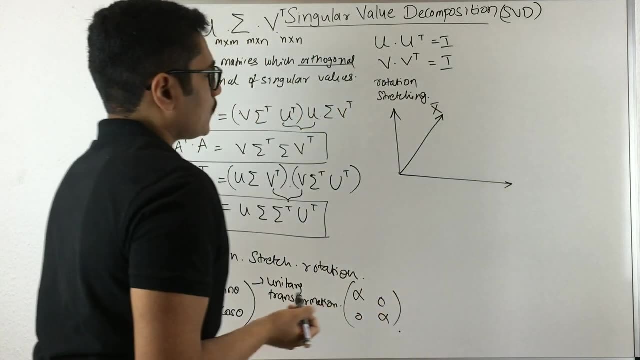 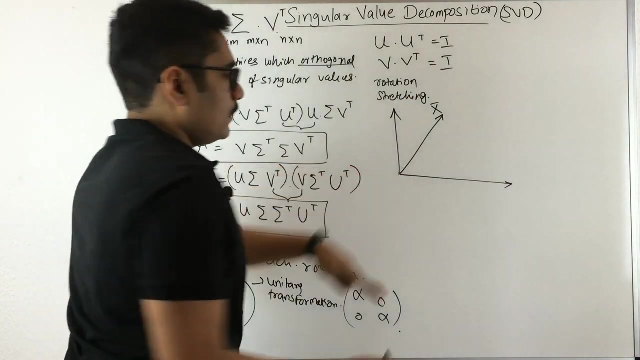 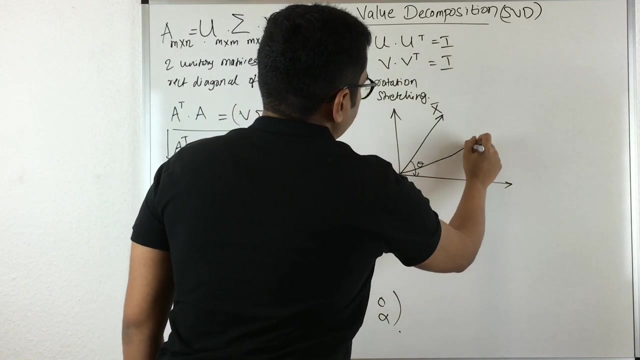 so, geometrically, if we want to represent, say, for example, we are considering some vector, or say we have some x vector Now. Now, according to this definition, what happens is you will just rotate this x vector down this way with some angle theta. So what you obtain is: you have this. so this length is 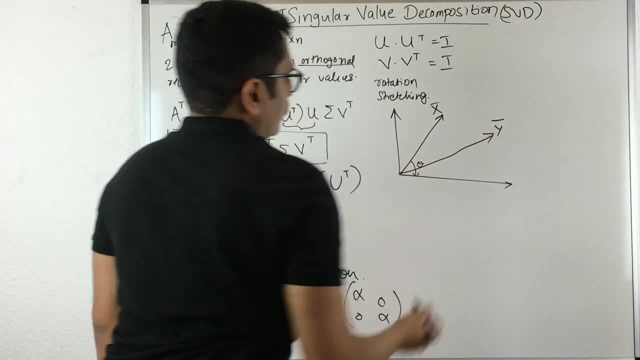 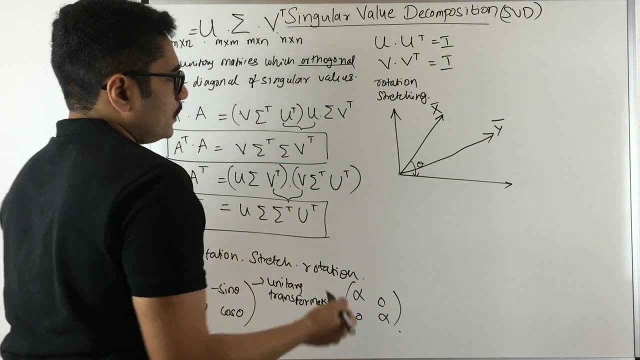 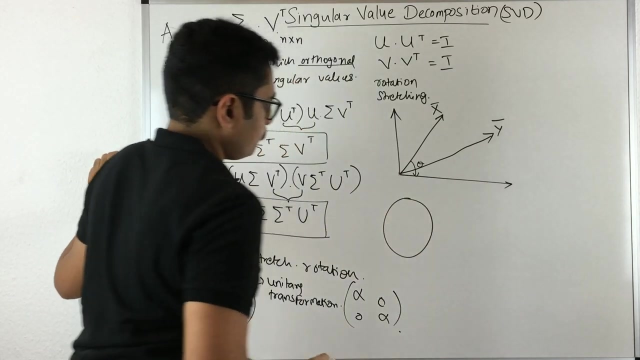 not equal to this. So say this is a y bar. So since you have rotated this x here and you have stretched so that essentially becomes your SVD now. Now let's take one more example. say you have a circle like this. So in two dimension, 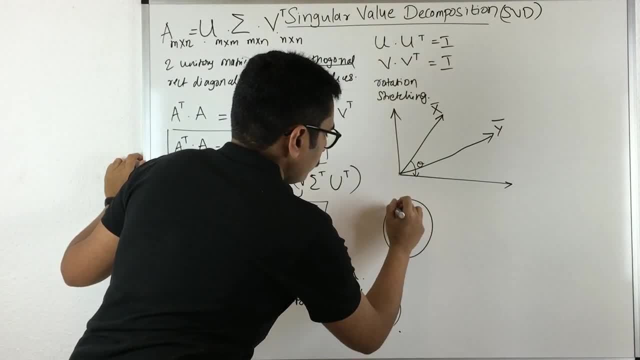 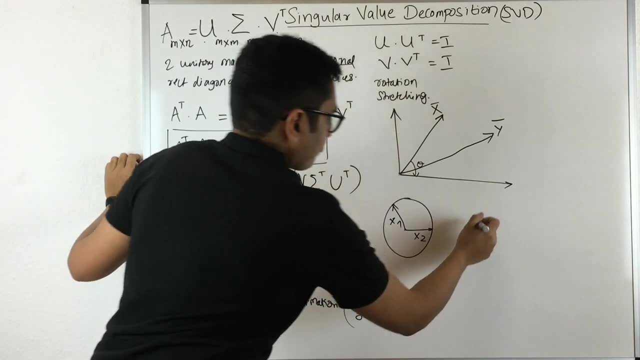 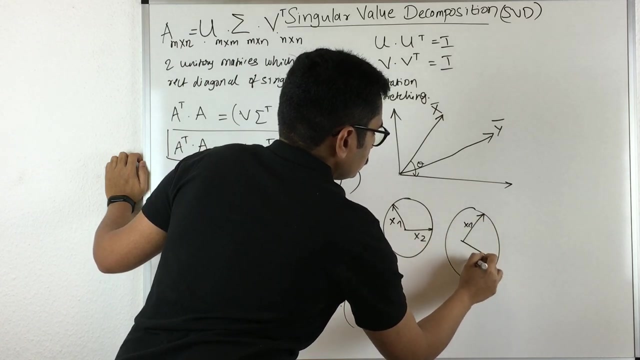 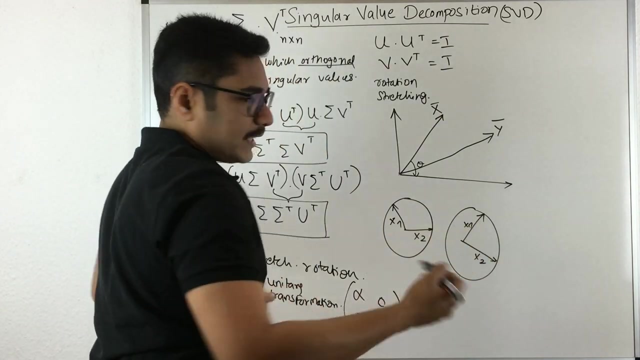 this becomes a circle. now the circle will have, say, two vectors, such as x1 and x2. now if you rotate this vector at some particular axis, say, you have this tilted over this direction, but this effect is not that significant. So what you do is you just stretch it. So when you stretch this, it becomes an ellipse. 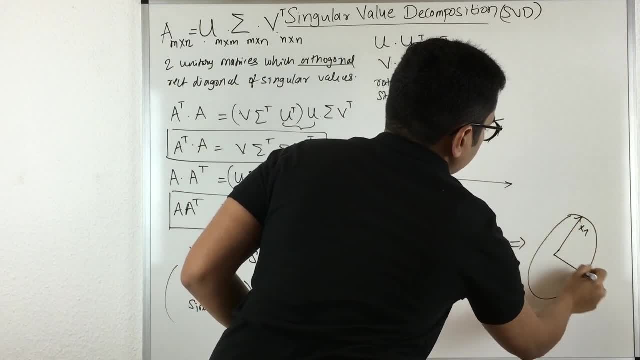 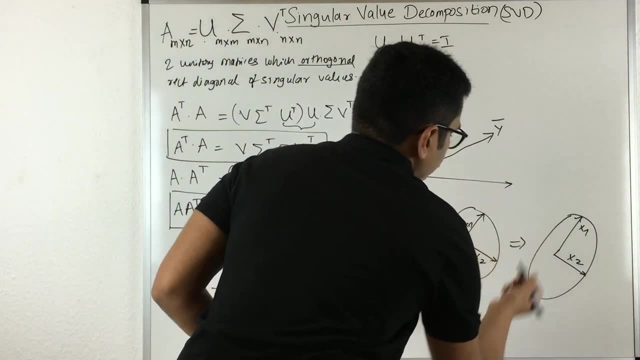 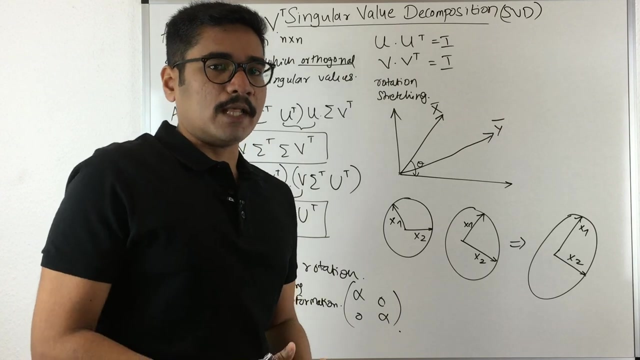 in this way. So this is your X 1 and this is your X 2.. So this is what we basically do in singular value decomposition. So now what we want to do is we need to apply to our different algorithms so that it will reduce our matrix a into three. 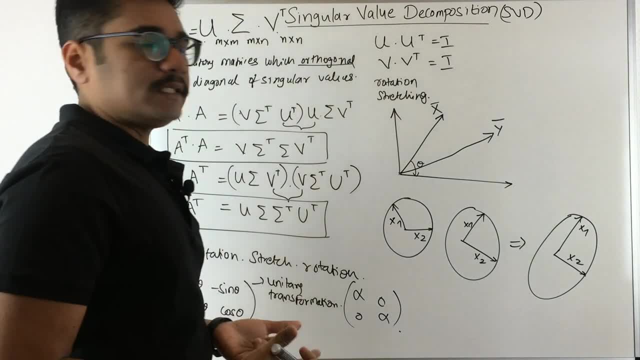 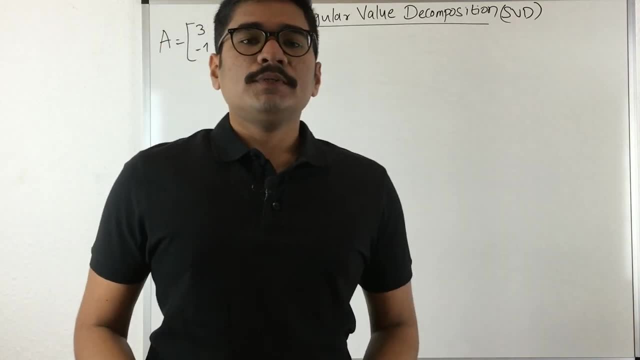 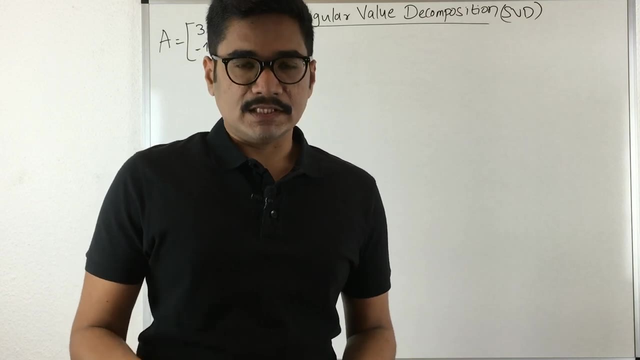 three of this components. So for that, let's take one example regarding how we'll solve the SVD. So now what we do is we'll just illustrate the concept of SVD in terms of matrices and how different matrix multiplication is done and what all are the various components that 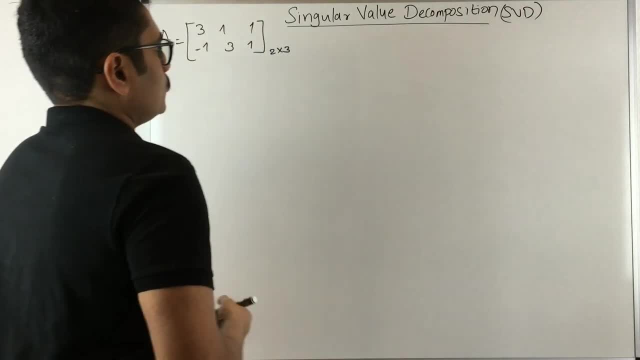 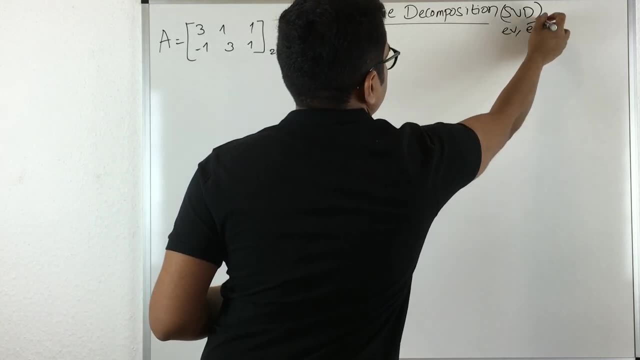 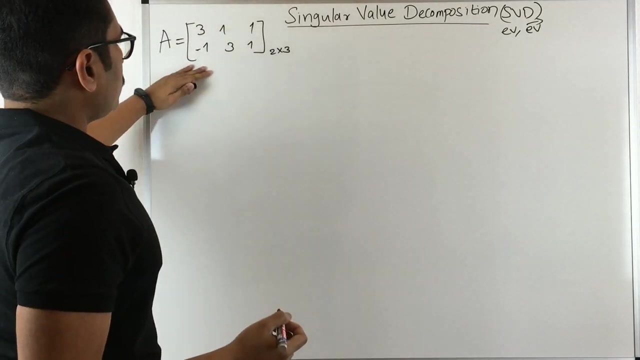 we take into considerations when we do the SVD. So whenever we do SVD, we have to compute two things, that is, eigenvalues and eigenvectors, like we saw in the principal component analysis. Now for this, just consider this matrix A. So this is a 2 cross 3 matrix. Now what we 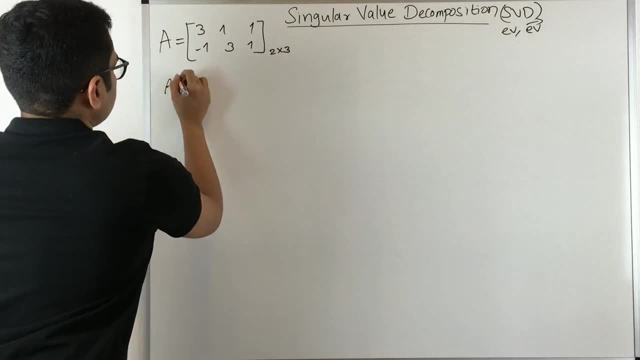 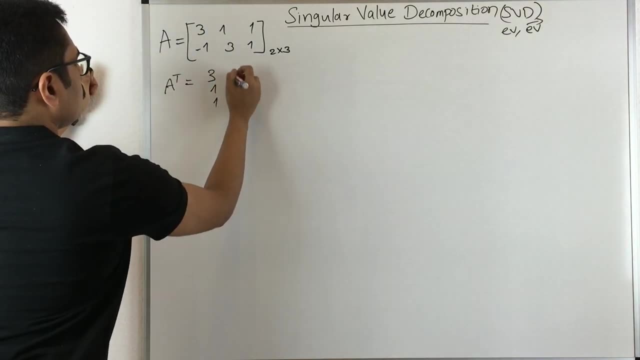 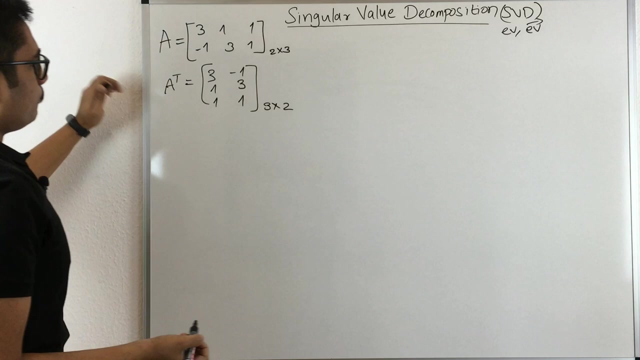 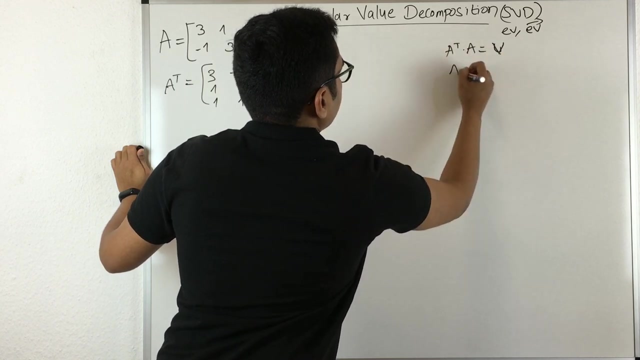 need to have is we need to have A transpose of this. So how do we write the transpose? rows are converted to columns, So you have 3, 1, 1 minus 1, 3 and 1.. So now this becomes a 3 row and 2 column matrix. now from our definition We know that A transpose, A is V and A A transpose. 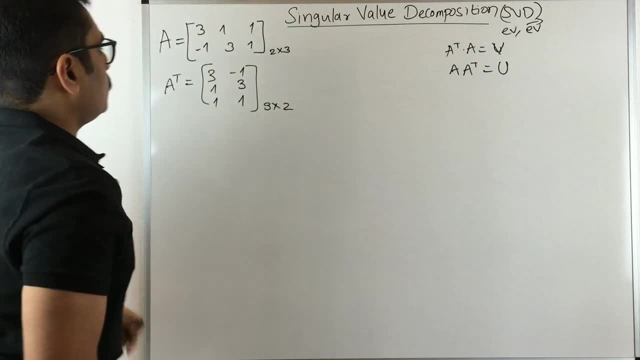 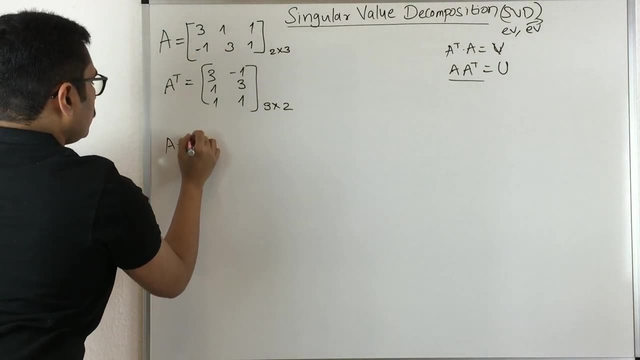 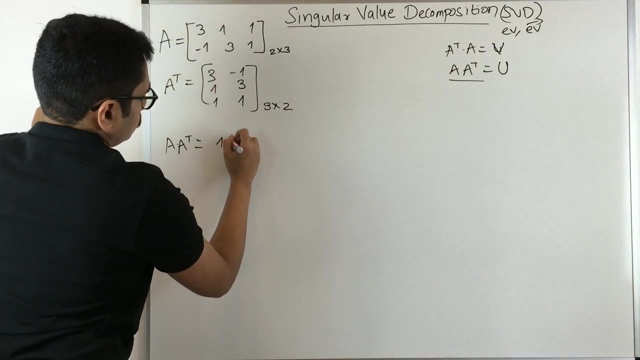 is U. So we want to have this. matrix is now first we do that is A and A transpose. So when we do A and A transpose, what we achieve is we have to do the matrix multiplication. So in the same way, what we achieve is 11: 1.. 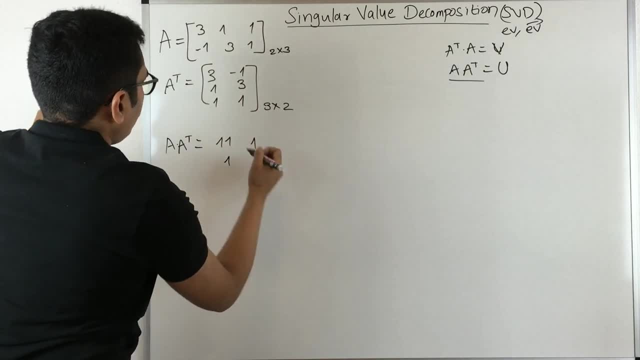 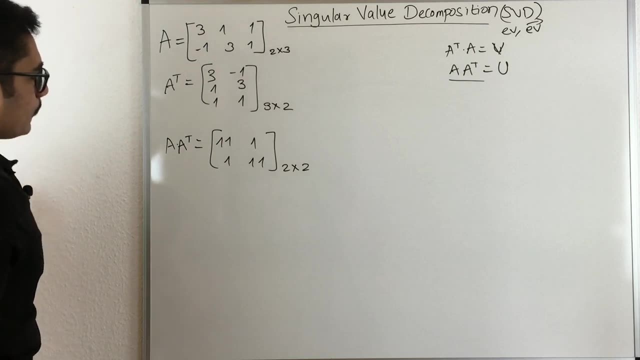 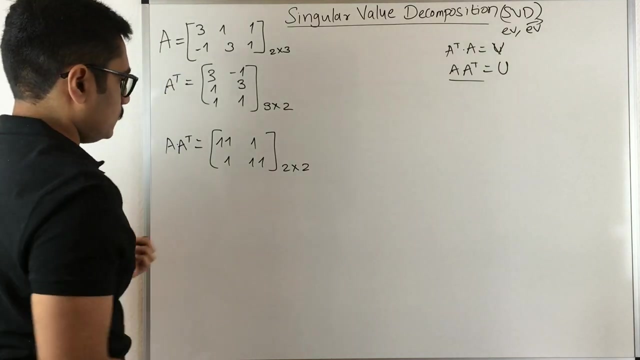 Then you have 1 and 11. So the resultant is a 2 x 2 matrix that we achieved. Now, in order to find the eigenvalues and eigenvectors, what we need to do is we need to write the characteristic equation for this. So how do we write the characteristic equation? So, in terms of matrix, 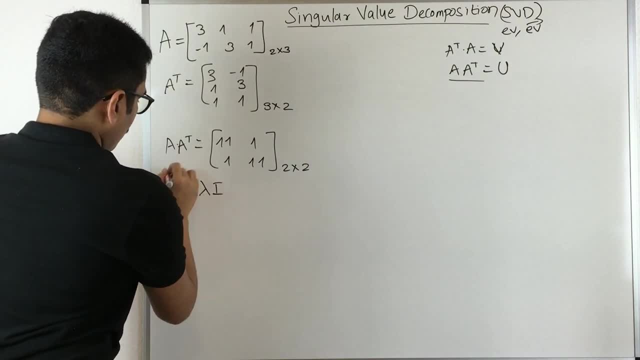 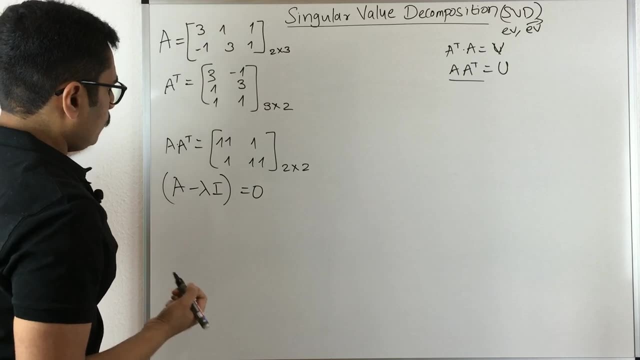 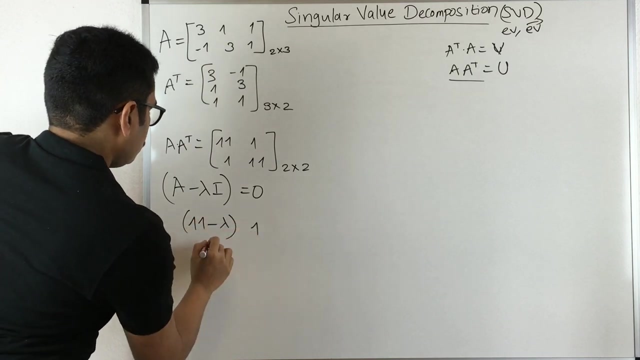 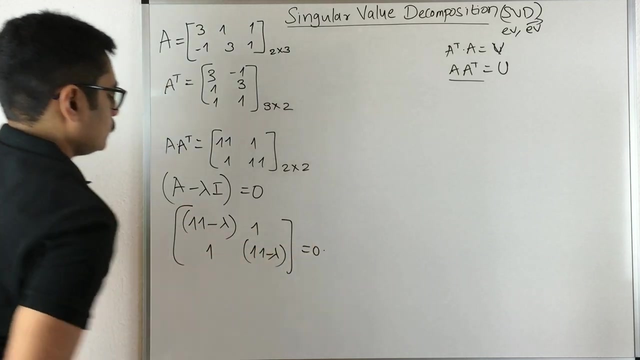 we have A minus lambda I X threshold equals 0. So you want to write in this way. So what we basically do is we just subtract from the diagonal 11 minus Lambda, 1, 11 minus Lambda. So now, this is our equation. now, from this will find the values for lambdas. 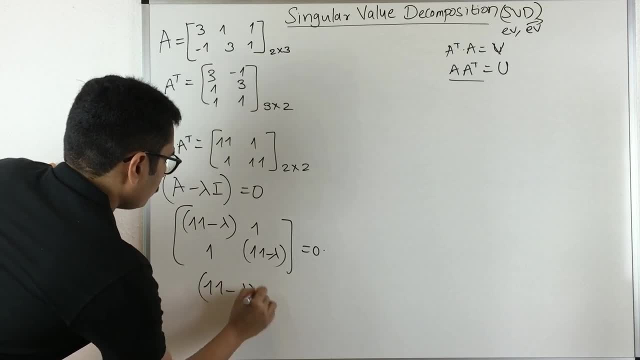 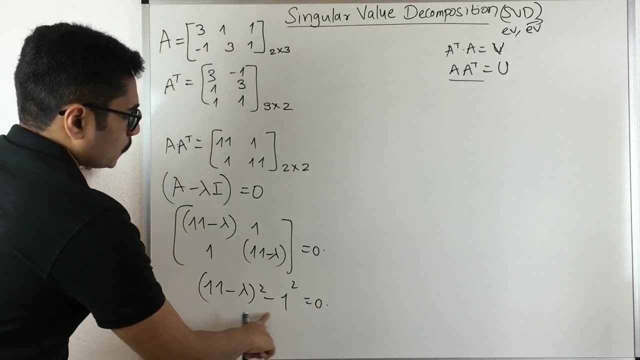 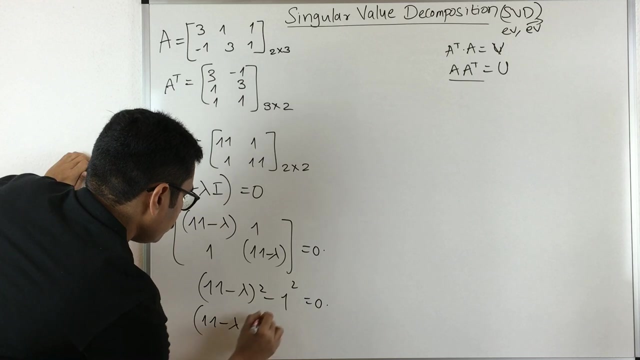 So how do you compute this? 11 minus lambda square minus 1 square. So, if you remember, this is of the form a square minus b square, which is a plus b and a minus b. So that is a plus b and a minus b, which is equal to 0.. 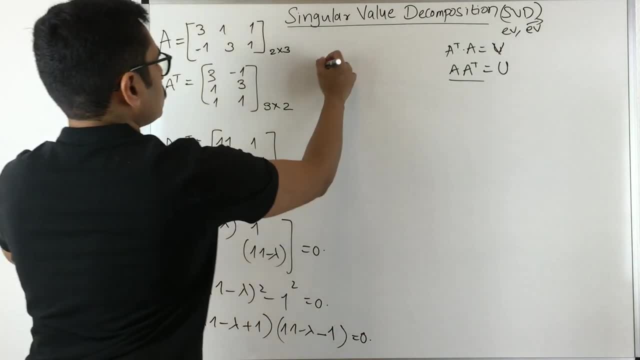 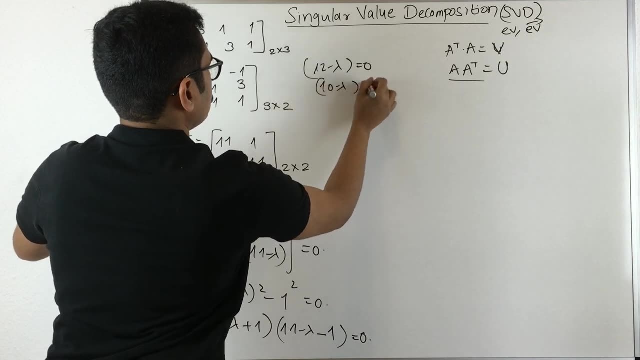 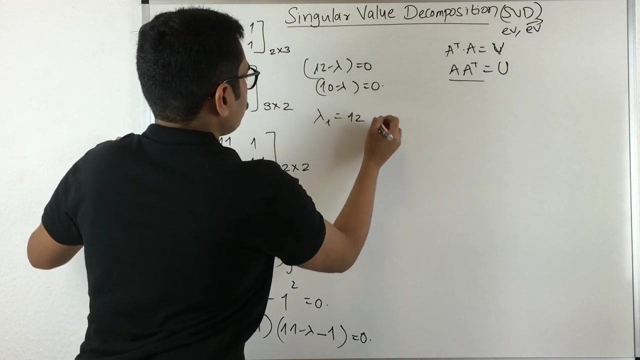 So if you solve for this, you have: that is 12 minus lambda is equal to 0, and you have 10 minus lambda is equal to 0. So you have 2. So you have 2 values for lambda basically. So the first value of lambda is 12 and the second value for lambda is 10.. 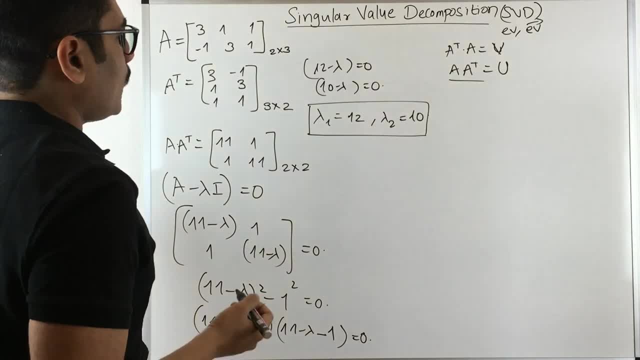 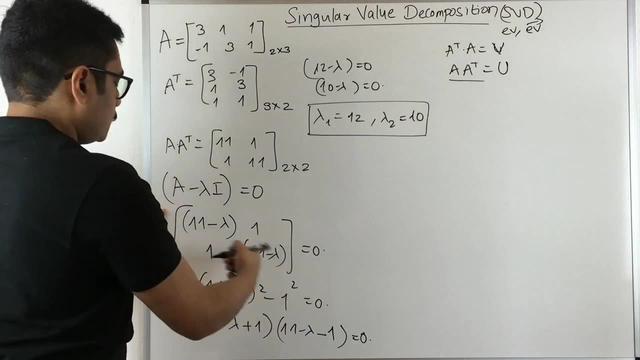 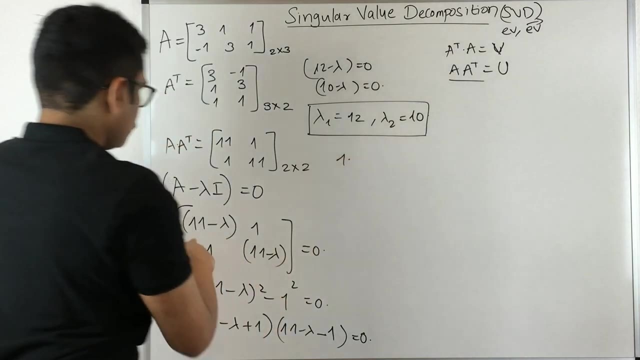 So you get these two eigenvalues. now you want to find the eigenvectors of this. So for that, what you basically do is you put into this equation, that is, you substitute for this value. So first you put lambda 2 and then lambda 1, so you have, that is 11 minus 10, that is. 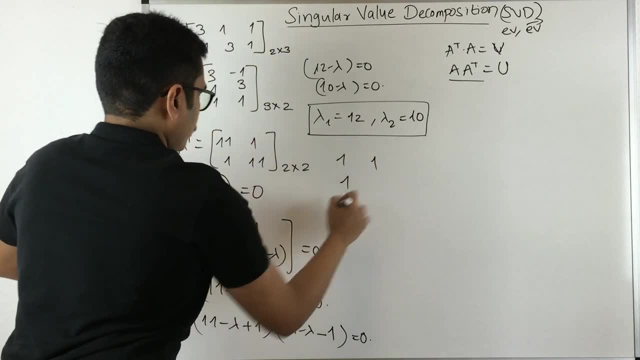 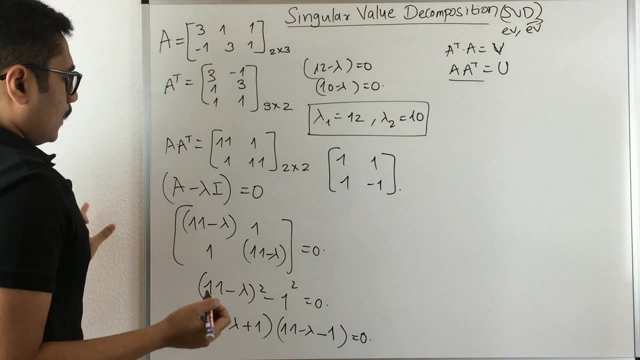 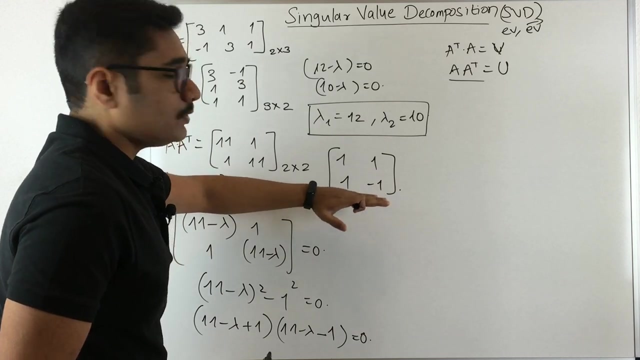 1.. Then you have this way, but here you have 11 minus 12, that is, minus 1.. Now, this is just what we obtained, the eigenvectors. But what you need to do is you need to do the orthogonalization of this particular matrix. 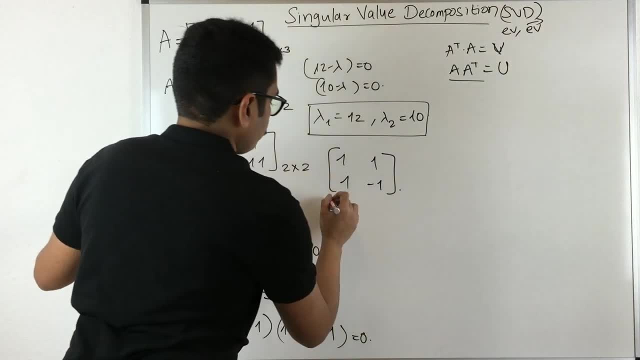 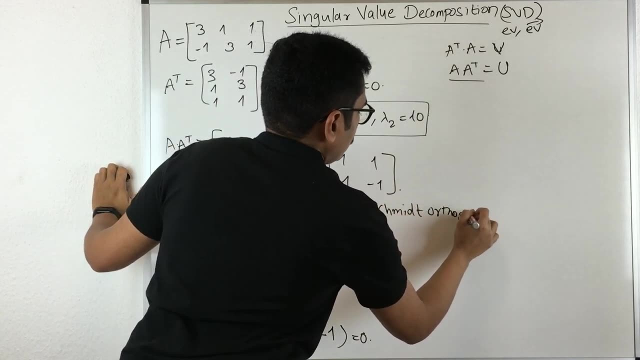 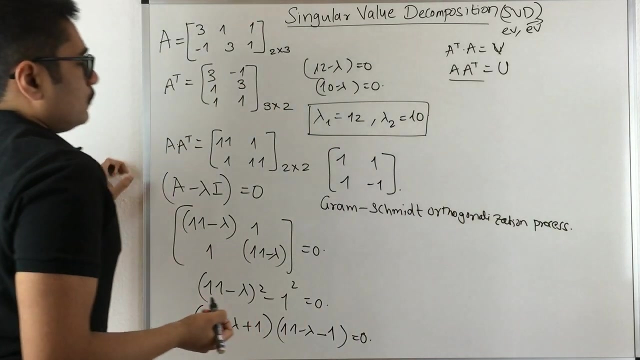 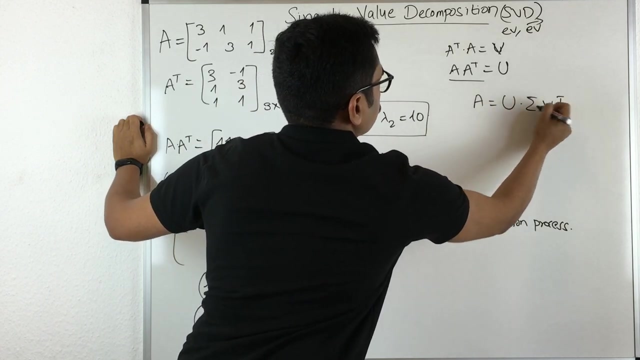 Now that orthogonalization is done with the help of Graham Schmidt orthogonalization Process. So, since what we basically do is we have this format, that is, a is represented in u Sigma and B transpose, So you need to have the first and the third matrix in orthogonal form. 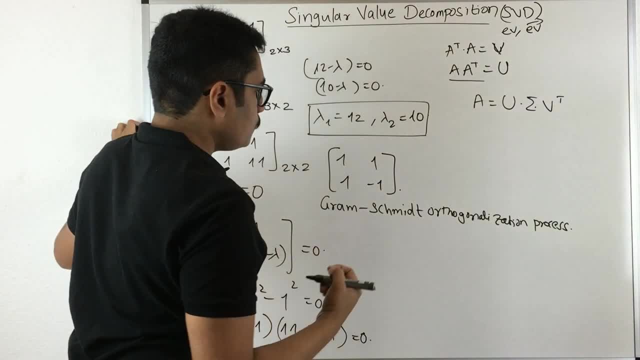 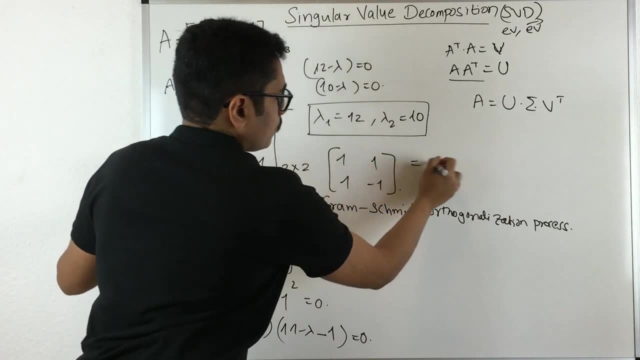 So that's why we are doing this orthogonalization process. So how do you do this? We just compute the length of each of this. So if you just compute the, that is square root, Okay, Square root of 1 square plus 1 square, and here you have square root of 1 square plus. 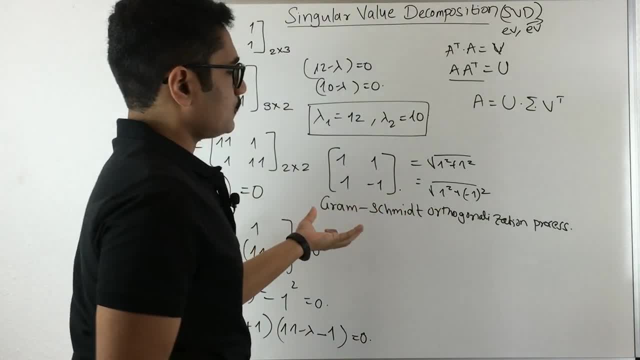 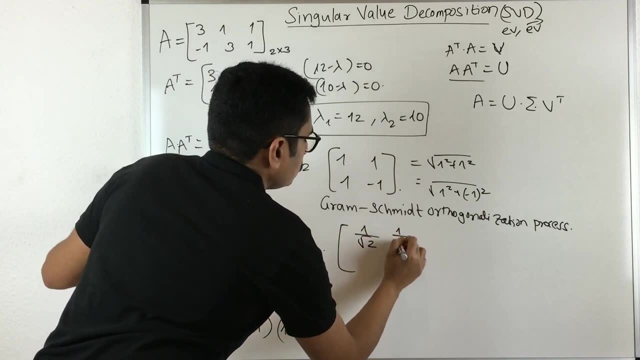 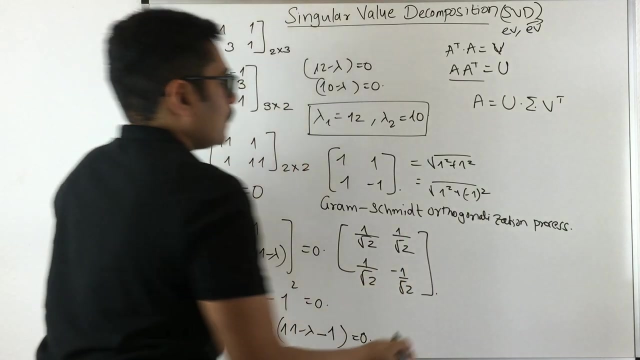 minus 1 square, So you have the length throughout this as root 2.. So what you do is you just divided by the length 1 upon root 2 and minus 1 upon root 2.. So this gives our u matrix. So this is our u matrix. 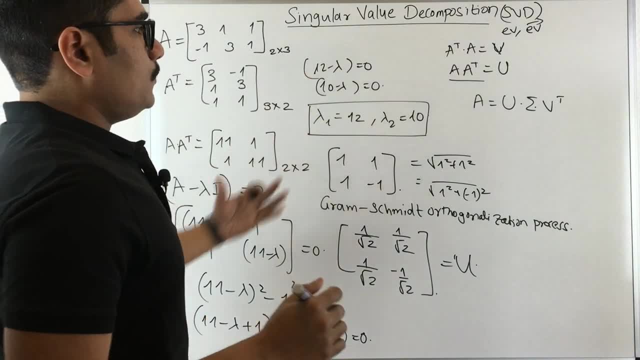 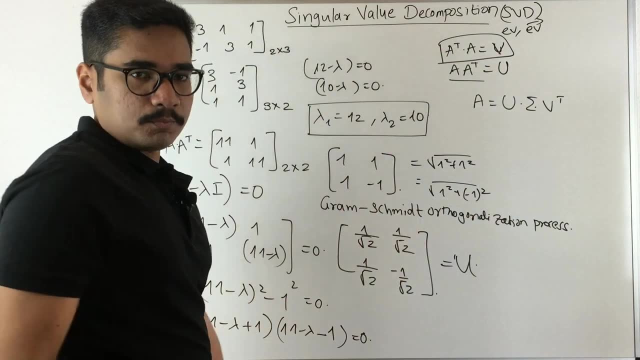 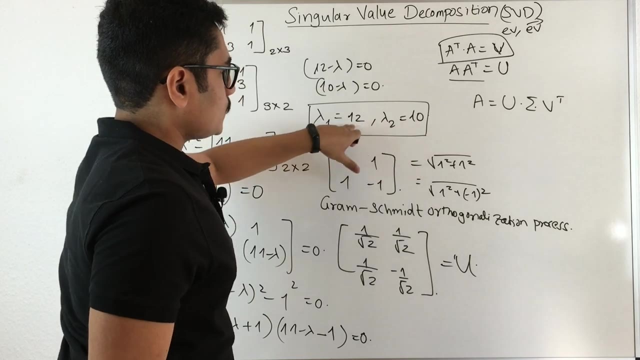 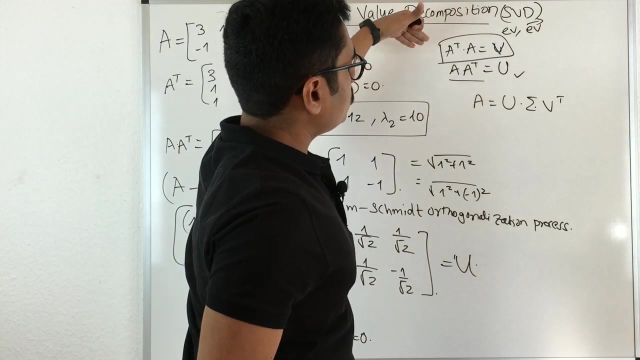 Now So v matrix. first we need to compute by using this identity equation and then thereafter we shall take the transpose and then we'll finally find the Sigma. So these are basically two singular values, which are unique, that you obtain, when you considered this operation now from similar when we compute this, a transpose and a you. 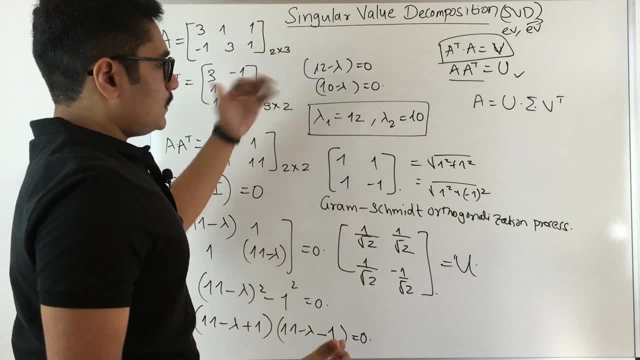 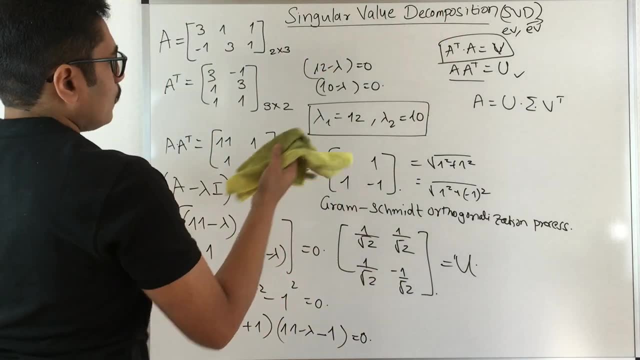 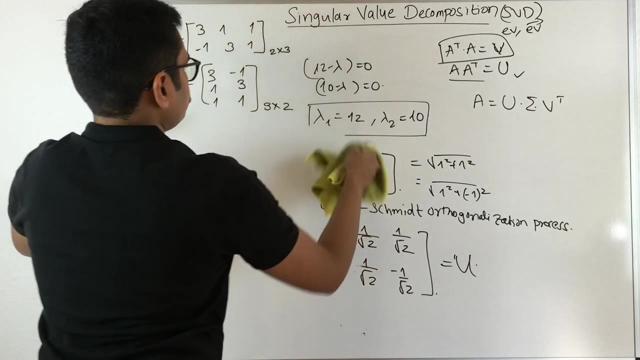 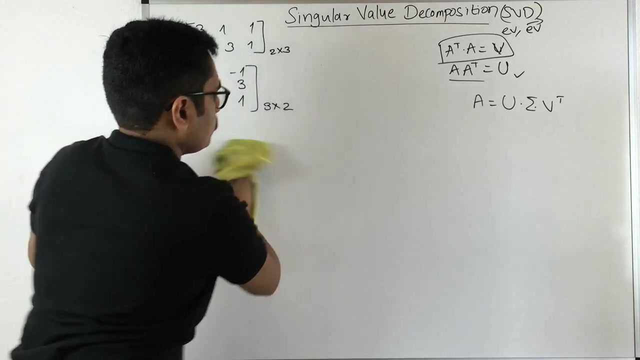 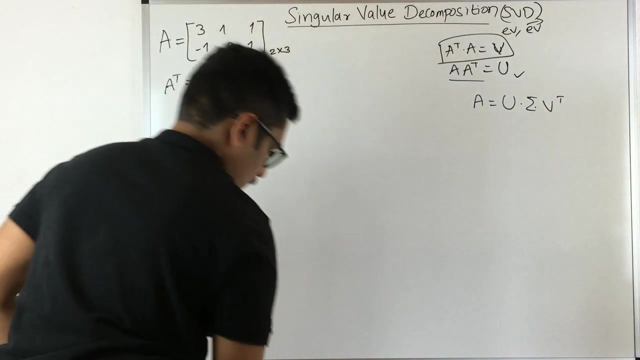 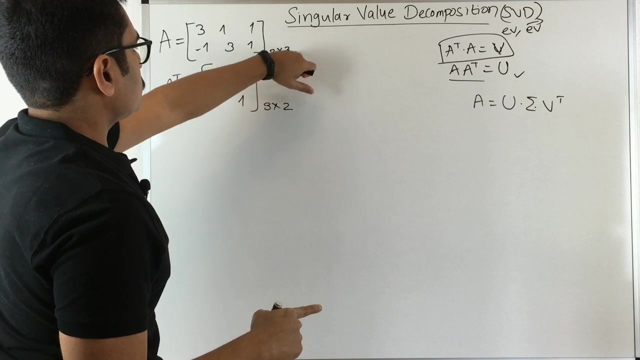 will get some sort of values, but we will check whether it's different or not. So now what we do is we shall do the operation that this: a transpose and a for v. We Okay, Alright, Now we have this equation. now, when you just multiply with a transpose and a, this just reduces to a 3. 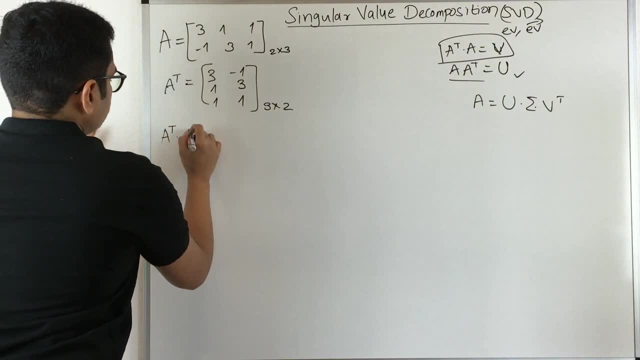 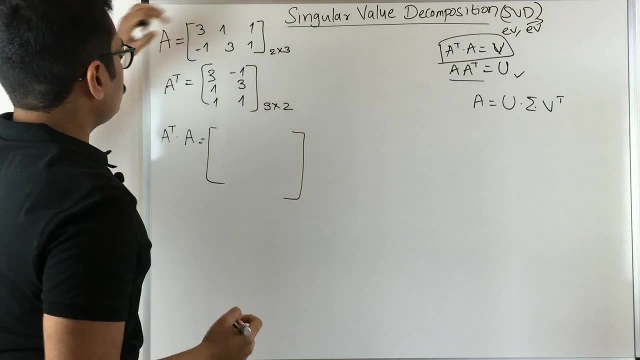 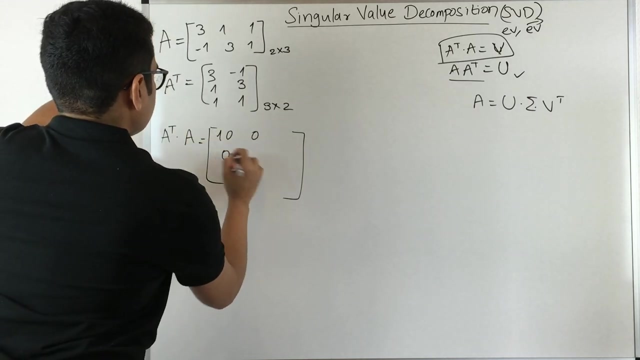 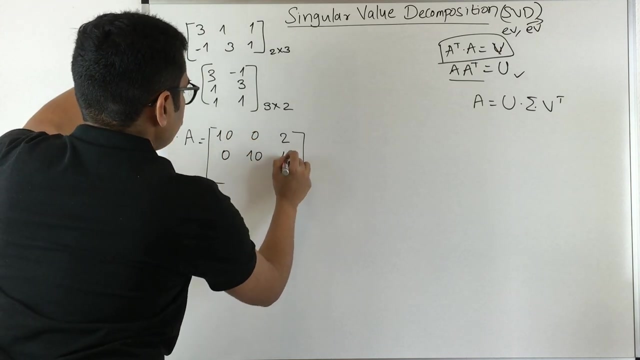 by 3 matrix. So when you do a transpose and a, you get this matrix in 3 by 3 form. So you get the values as 10- 0. Then you have 0- 10.. Then you have 2, then 4, then you have 2, 4 and. 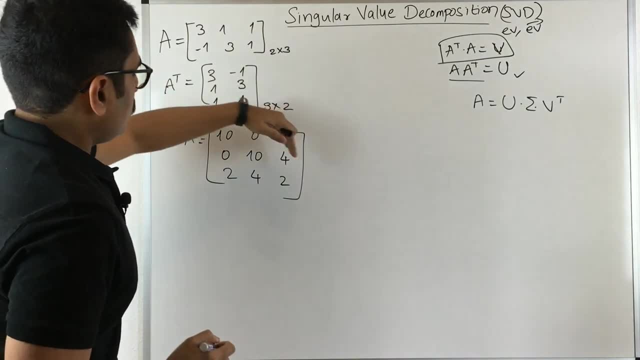 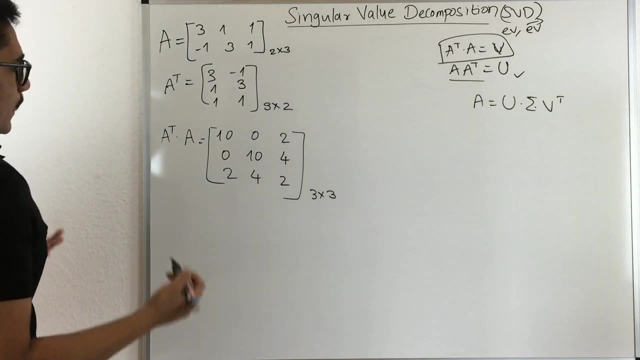 2. so this is how your 3 by 3 matrix would look like when you just multiply with this. as So, this is how your three by three matrix would look like when you just multiple And multiplying with this. Now again, what you need to do is you have to represent in the characteristic equation: 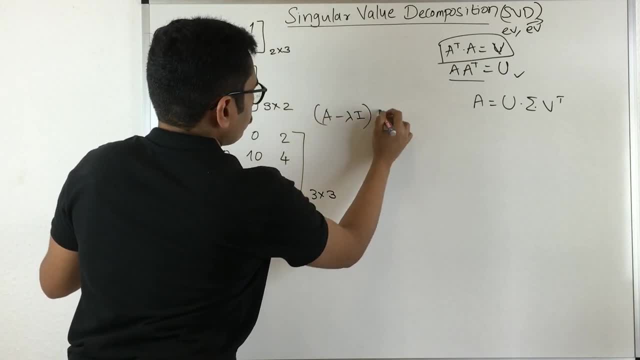 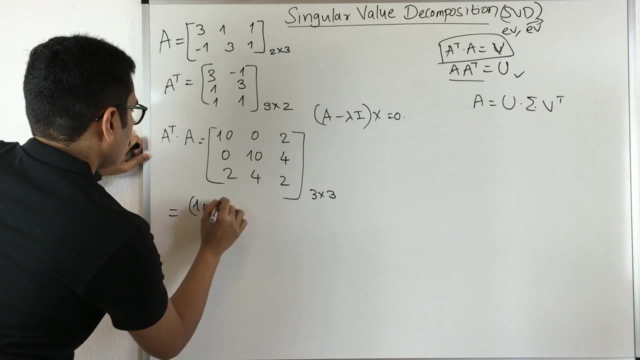 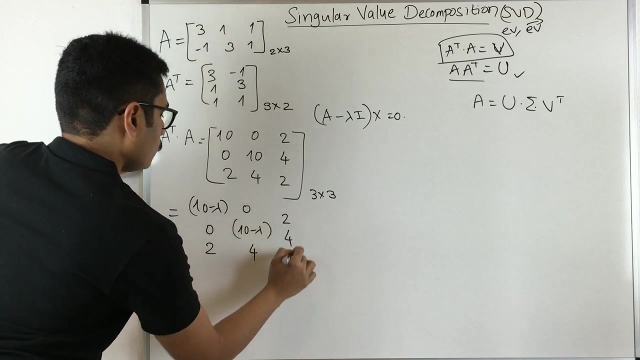 form. So that is a minus lambda. I, x is equal to 0.. So just subtract from the diagonals So that is 10 minus lambda, 0, 2, 0, 10 minus lambda, 4, 2, 4 and 2 minus lambda. Now finding: 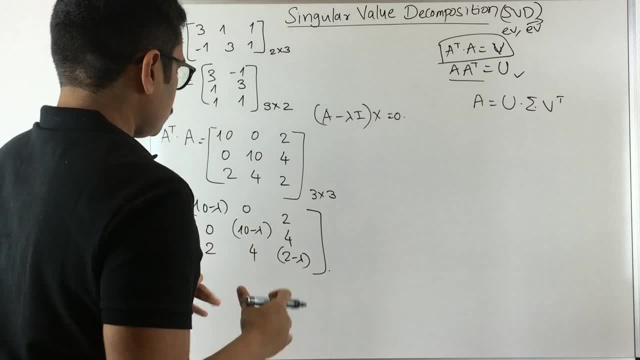 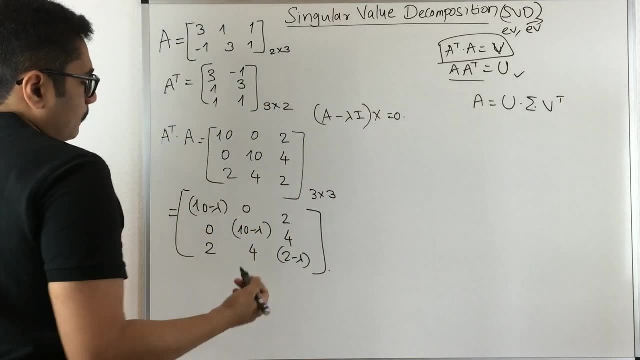 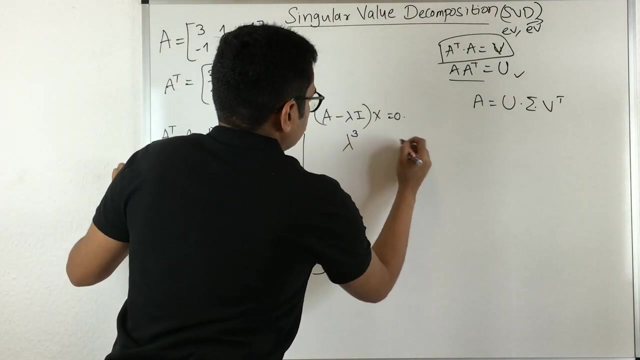 the roots of this is just a complicated form, but there is a shortcut technique which you can apply over this. So what you need to do, since it's a polynomial equation, so you have to write lambda cube. So since it's 3 by 3 matrix, you will write this equation, that is, lambda Square, then lambda. 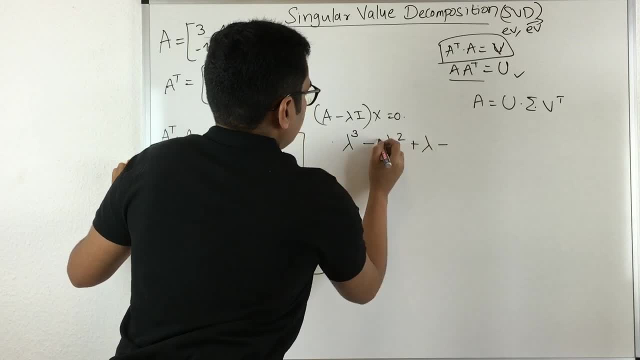 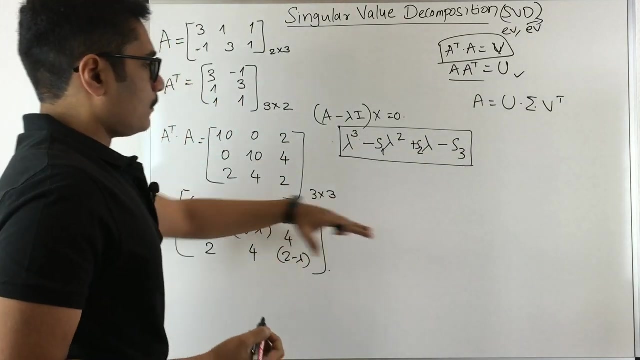 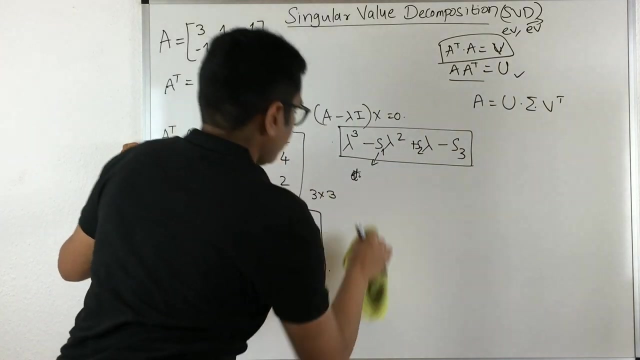 so plus, minus, plus and minus, and then you'll just compute three values, that is, s 1, s 2 and 6.. and S3.. So this is just a shortcut technique in order to find and factorize this particular polynomial. So S1 here is nothing but the determinant. the S1 is the trace of this particular. 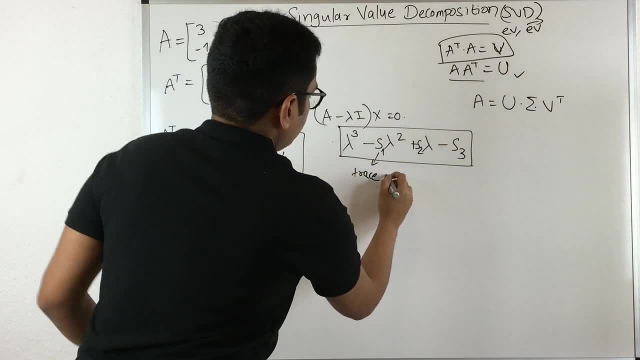 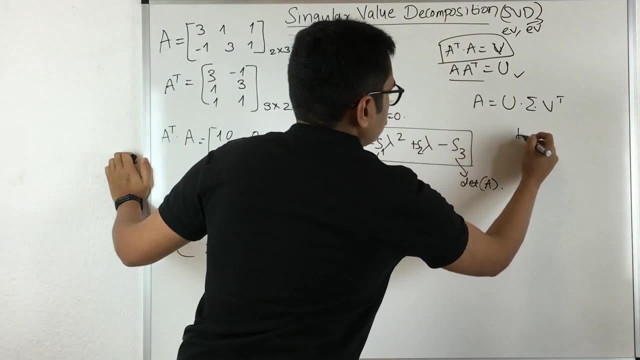 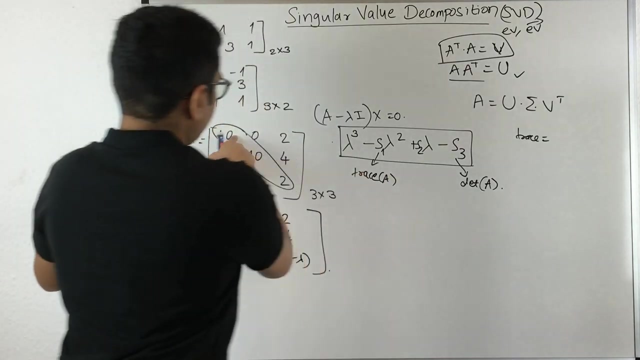 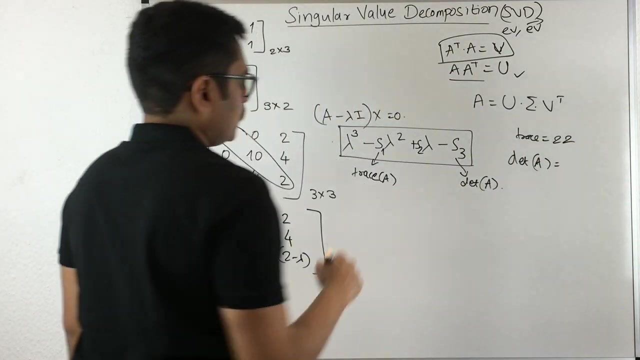 matrix. trace of a and S3 is your determinant of a. so trace is nothing but the sum of all the diagonal elements. that is some of all this. so you get 10 plus 10 plus 2, that is 22.. So you get the trace value as 22.. So now you have to find the determinant of this matrix. 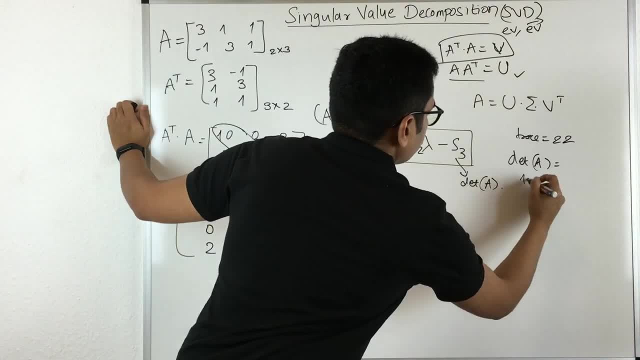 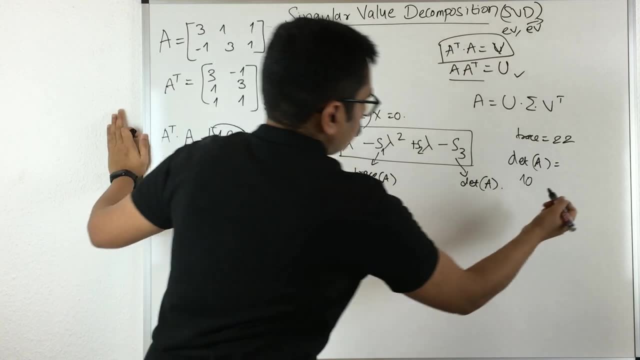 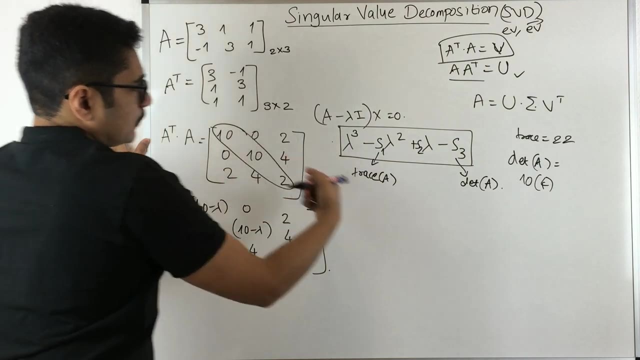 So how do you find the determinant? that is, you have ten and then you just multiply this portion, that is 10 to 20 minus 4, into 4, 16, that is 20 minus 16.. You get it as 4, and then the second term that is 0, and the third term that is 0, and the third term that is 0. So 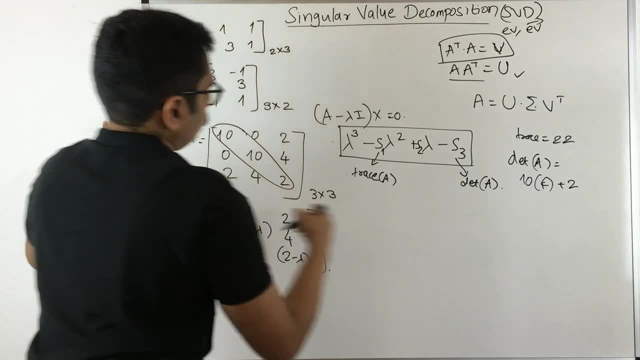 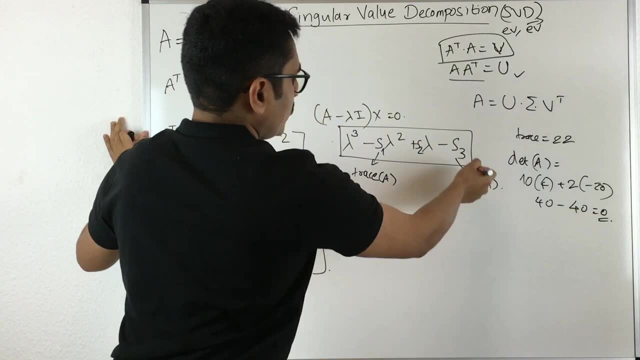 term is plus 2 into, you have minus 20.. So you get 40 minus 40, which is equal to 0.. So you are a determinant. that is, s3 is 0. now question comes: What is s2?? So s2 is nothing. 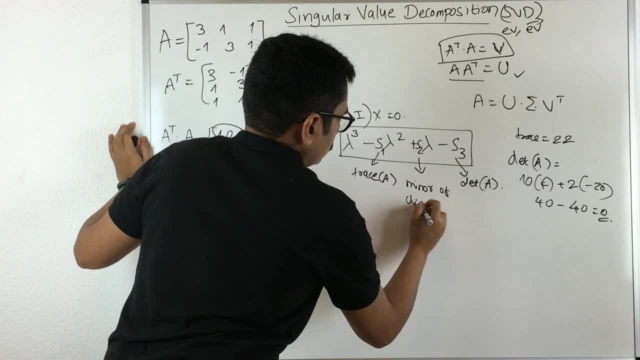 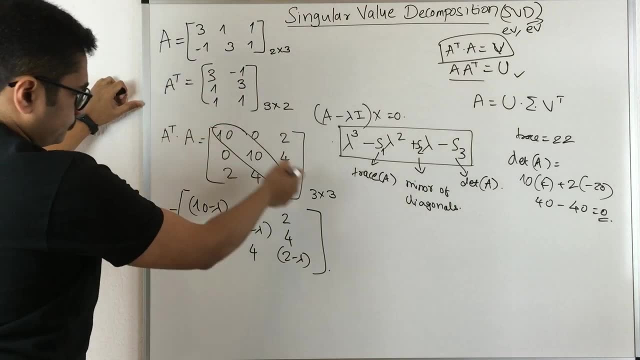 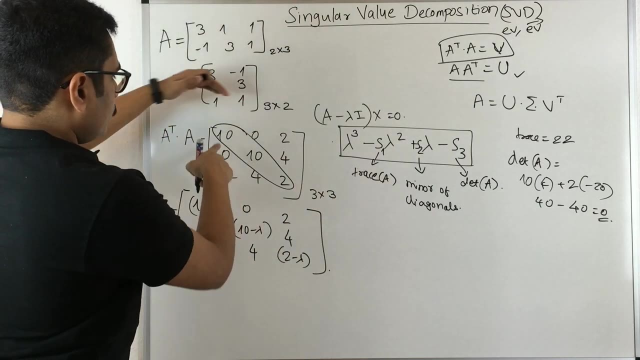 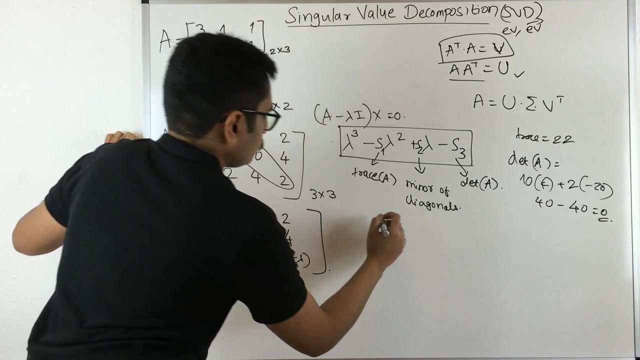 but the minor of diagonals, of this matrix, That is, these individual components. So you have to find the minors of this. So how do you compute the minors? So the very first minor is this: so you get this value as 20 minus 16, that is 4.. So you get the very first. 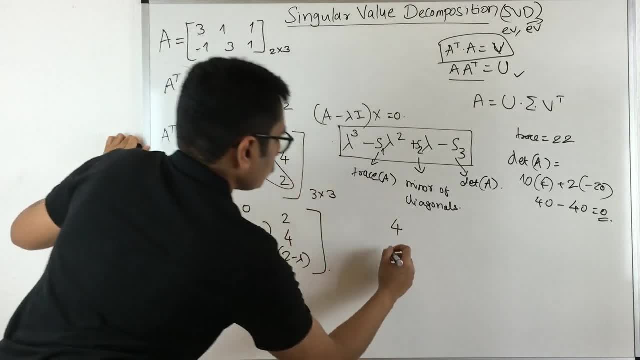 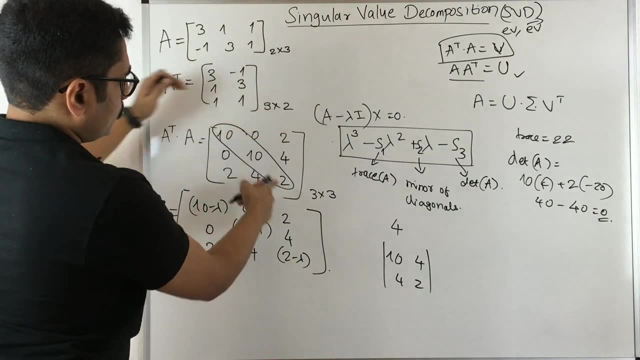 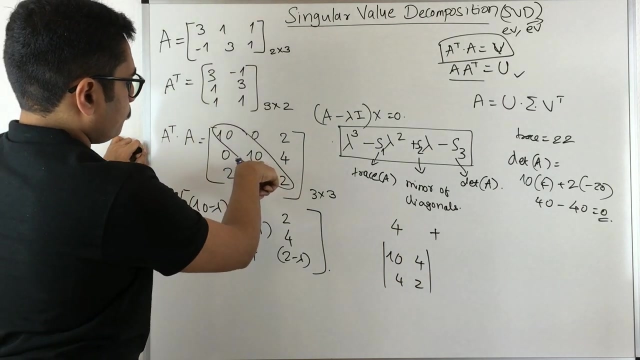 minor as 4.. So if you want to just write it so that becomes 10, 4, 4 and 2. so this is how we compute the minor this way, and then you have to add With this the second minor, that is this one that is diagonal. So you have all this: 10, 2, 2 and 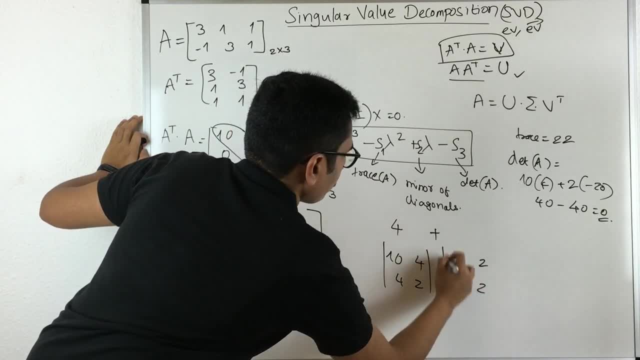 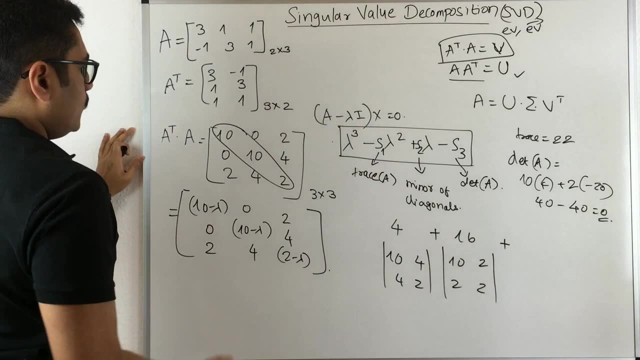 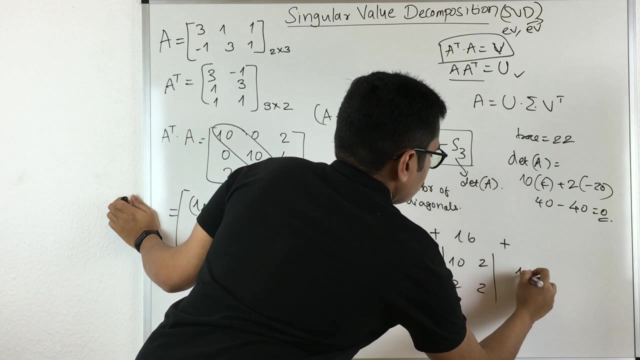 2, 10, 2, 2 and 2, so you get 20 minus 4, that is 16. then what you have is this: minor. So this is the third diagonal. So you want to find 10, 0, 0 and 10, so that is hundred minus. 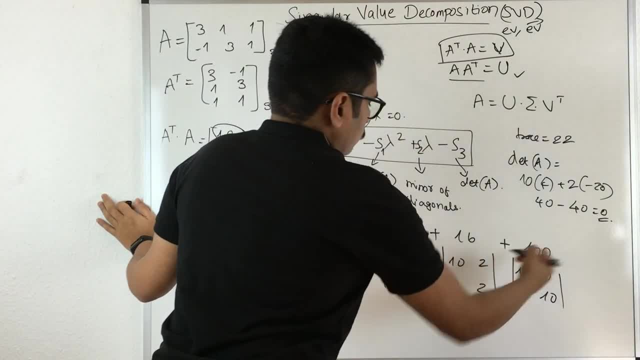 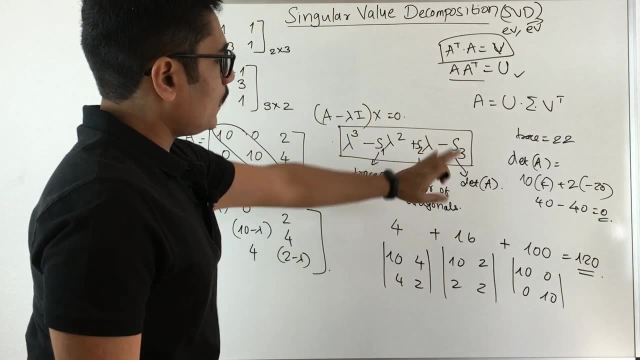 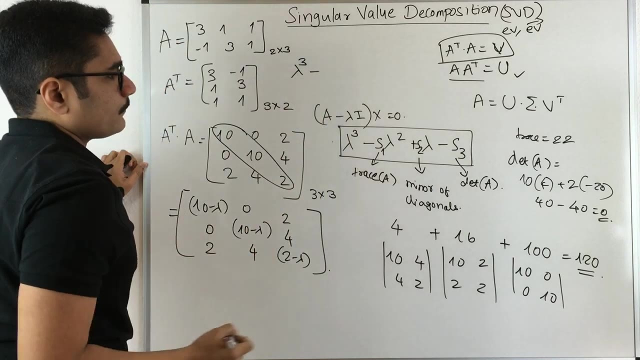 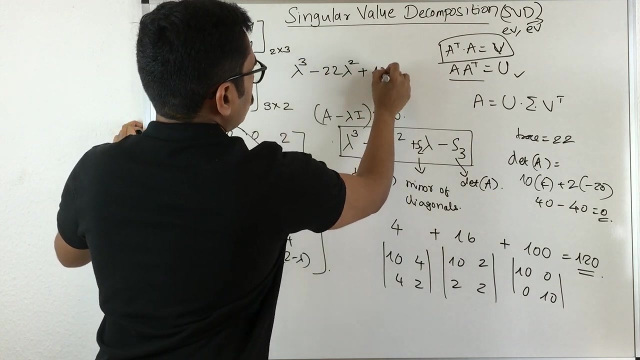 0, that is hundred. So now what you get is this value as 120.. So you have the s2 value as 120.. So now our final characteristic equation becomes: lambda cube minus our s1- that is, trace- was 22 lambda square plus 120 lambda, and this 10 is equal to 0.. So now we want to do the 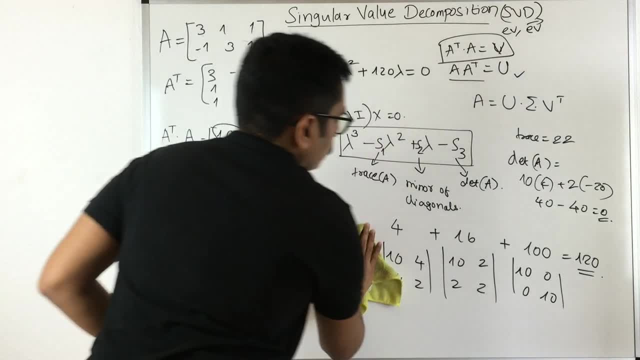 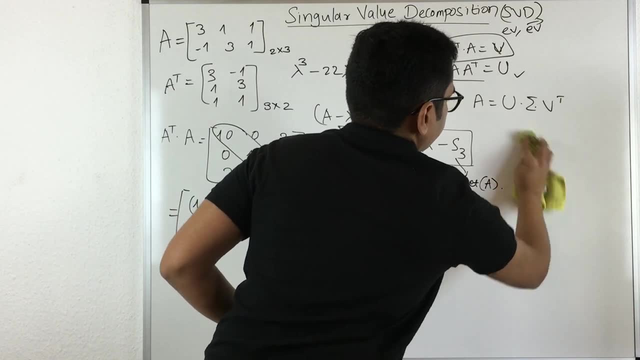 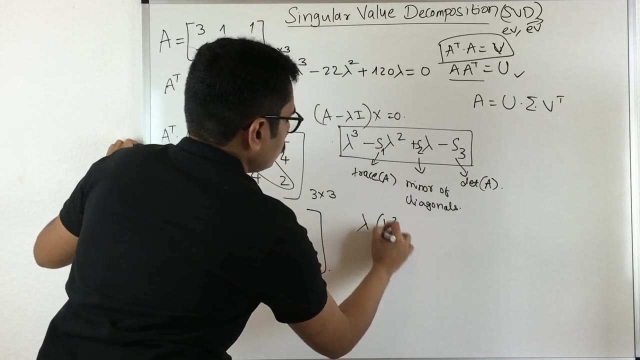 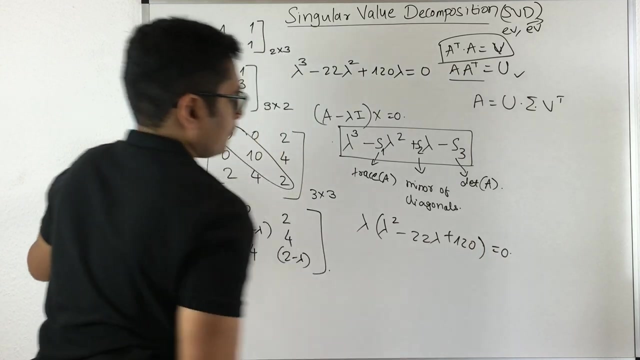 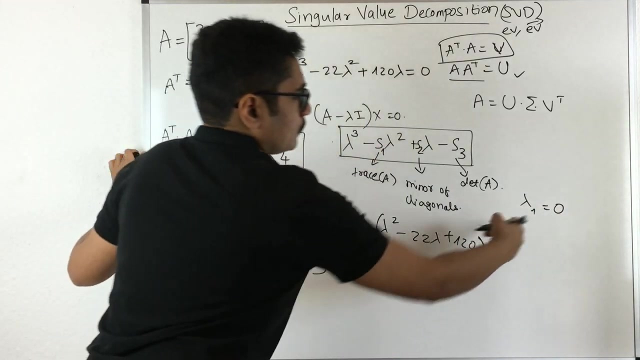 factorization of this, so that factorization is also very simple. So how do you compute the factors? So just take out 1 lambda out you have, plus 120 is equal to 0.. So the very first eigenvalue you have As 0, so just call it as lambda 1.. Now what you're left with lambda square minus 22 lambda. 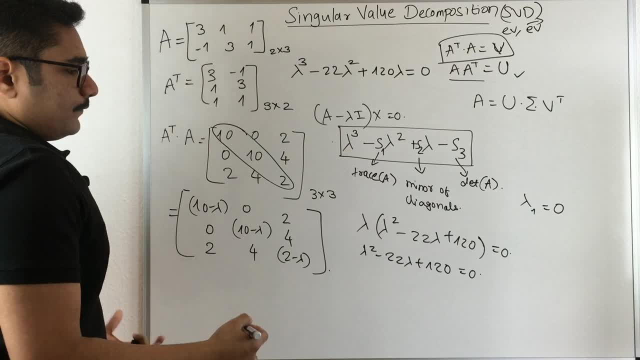 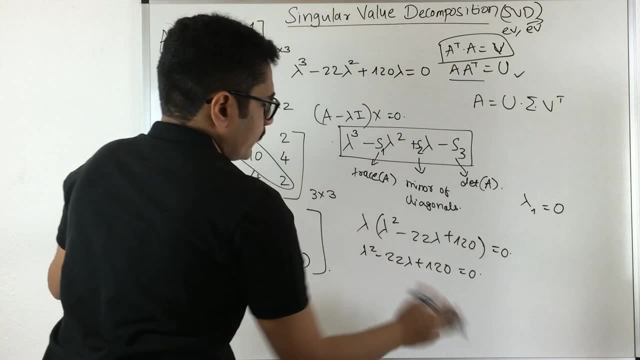 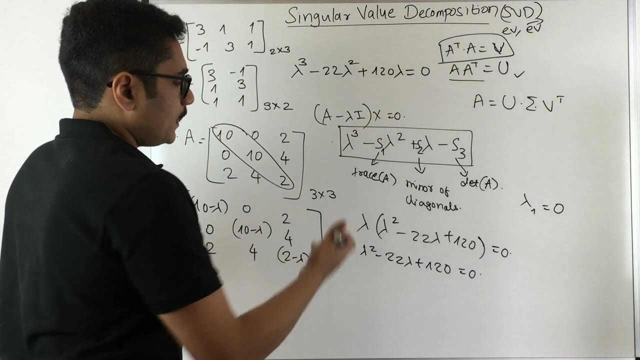 plus 120.. Now this is the basic factorization that we have learned in lower classes. just this, a small linear algebra which we do here. So we have to find the factors in such a way that when you just multiply you get the value as 120. But when you just add it up you get 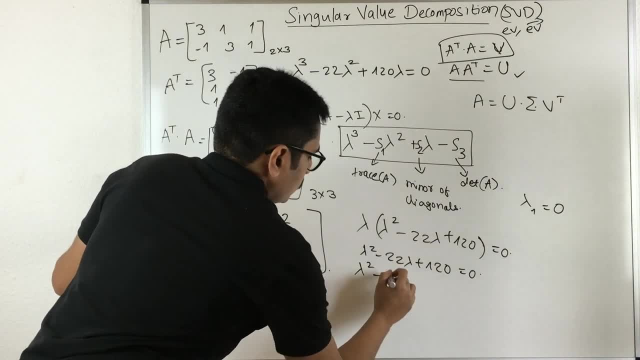 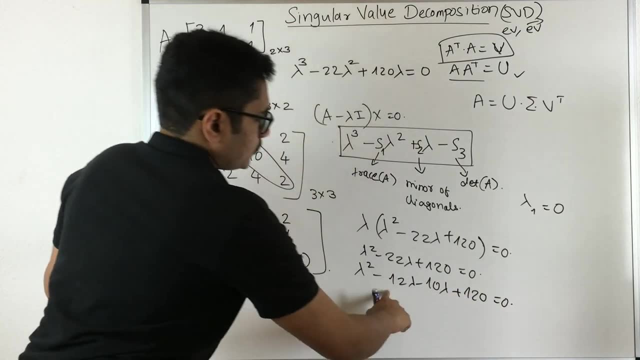 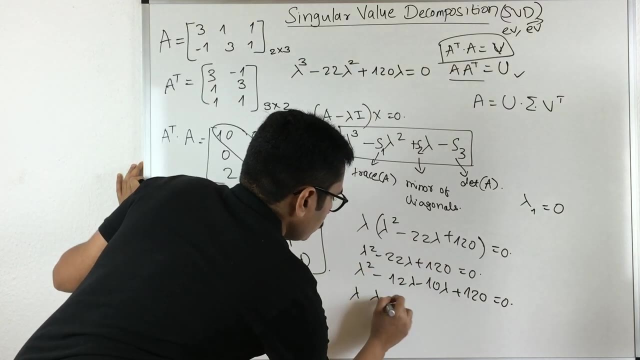 s minus 22.. So that is 12 lambda minus 10. lambda plus 120 is equal to 0.. So if you just multiply these two, you get 120. if you add the, you get minus 22. you take out lambda common from this minus 12 and you take. 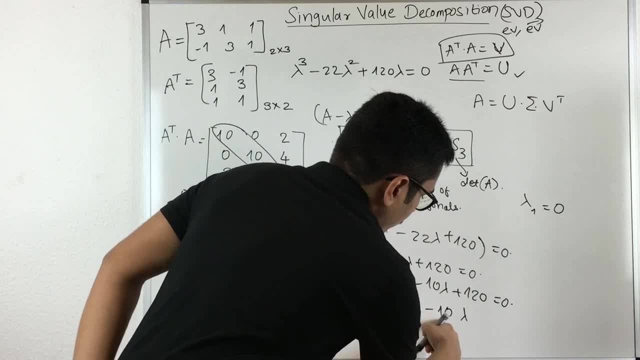 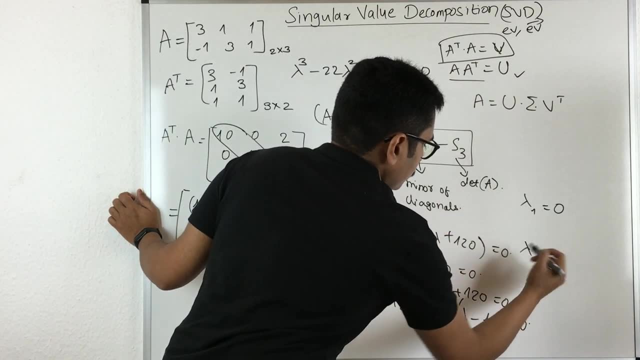 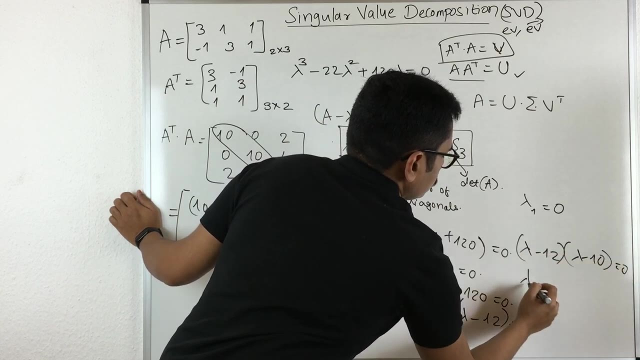 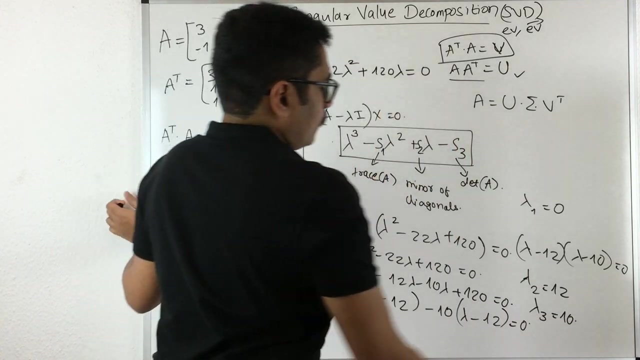 out minus 10 common. take minus 10 common inside the bracket, you have minus 12, which is equal to 0. So in the similar way, you have lambda minus 12 and you have lambda minus 10, both are equal to 0. So you get say the second value as lambda 12 and third value as 10.. 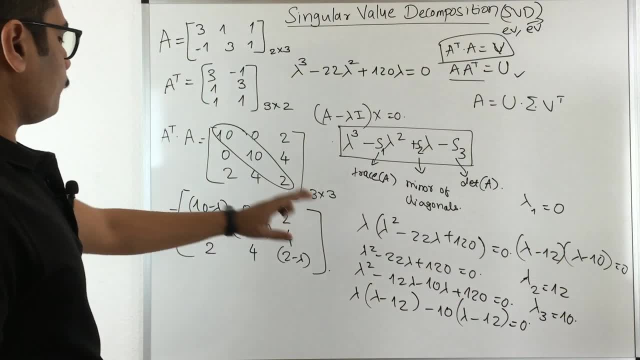 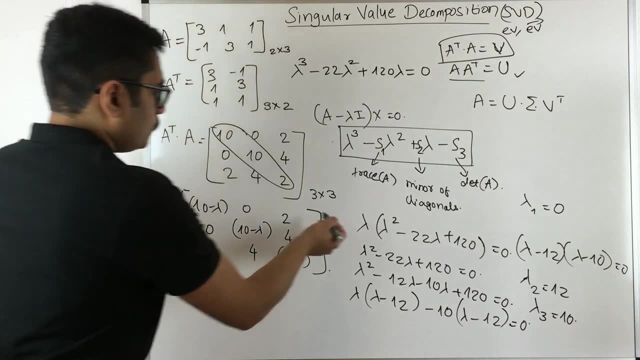 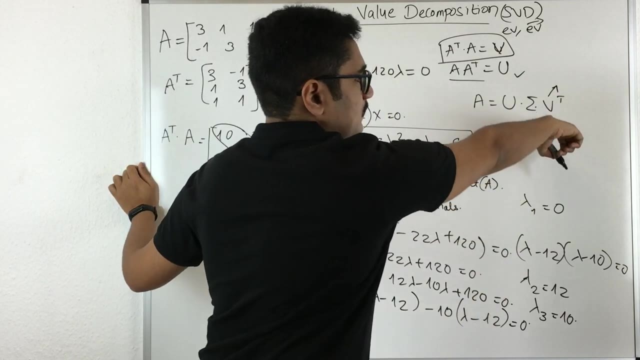 Now you have all these, now you want to plug in into this matrix so that you will get the individual values. So now what you have is you have this X, that is, column vector The. So, mind you, this V, that is, this orthogonal matrix, is in form like we have: V1 transpose. 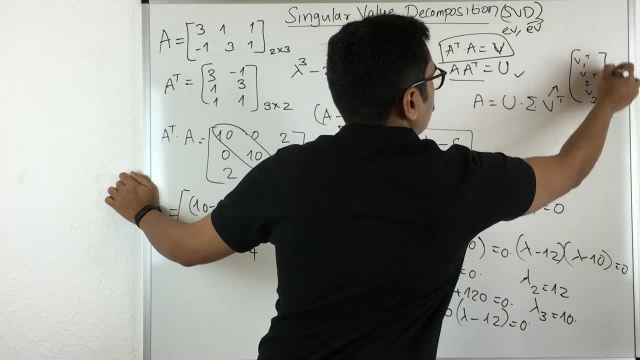 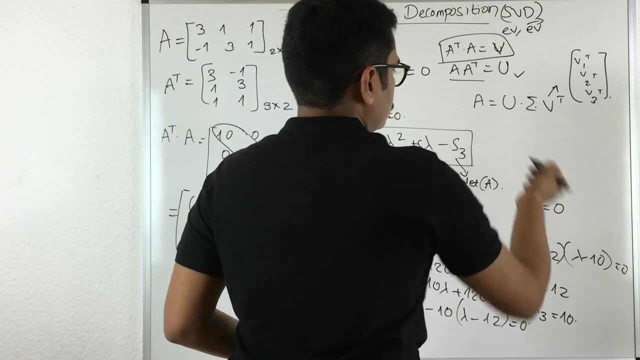 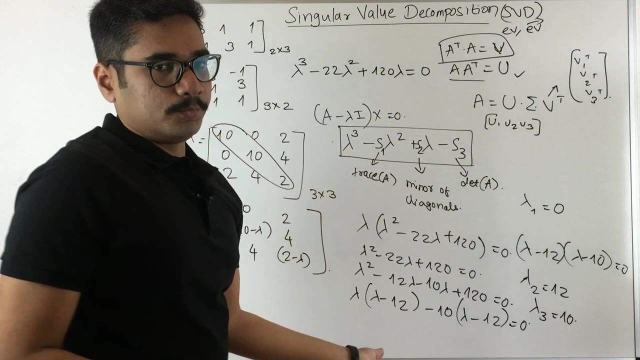 V2 transpose, V3 transpose. So this is a column vector. So if you have a row vector, you have to convert it into a column vector. and this U, this is orthogonal, This is not just a transpose. So you have U1, U2, U3 and these are just singular values that we'll see after computation of. 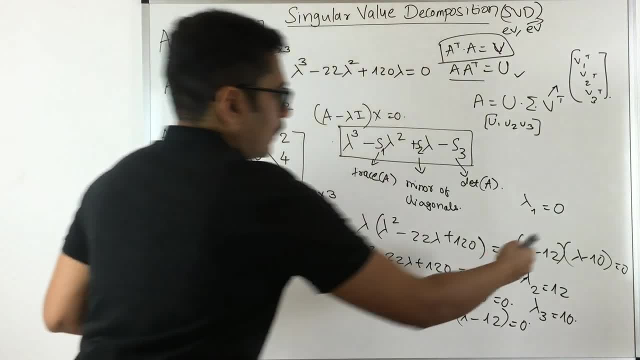 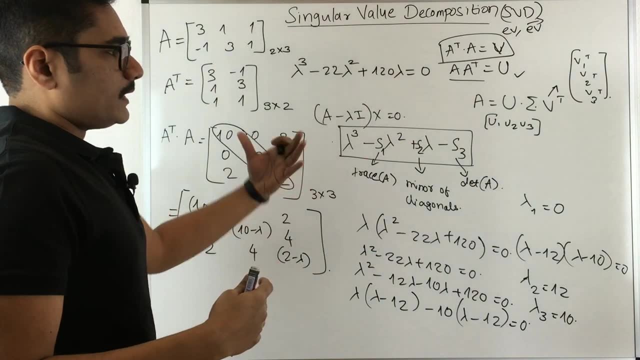 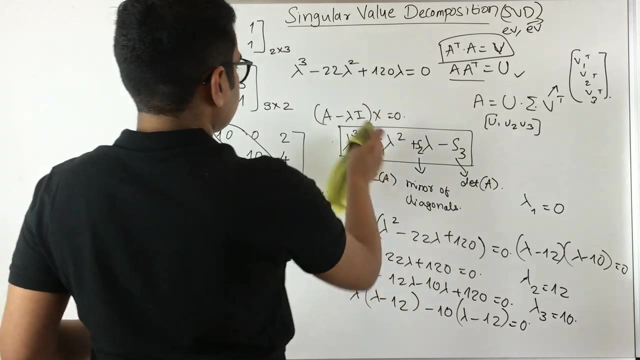 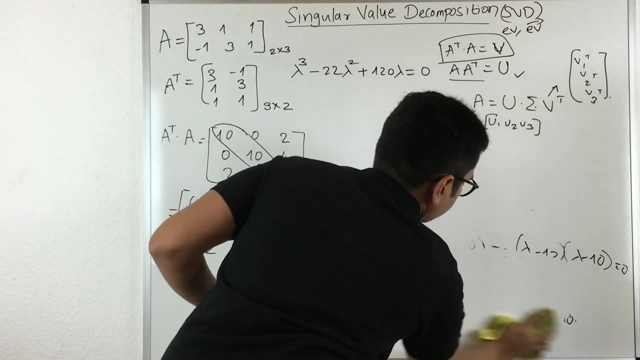 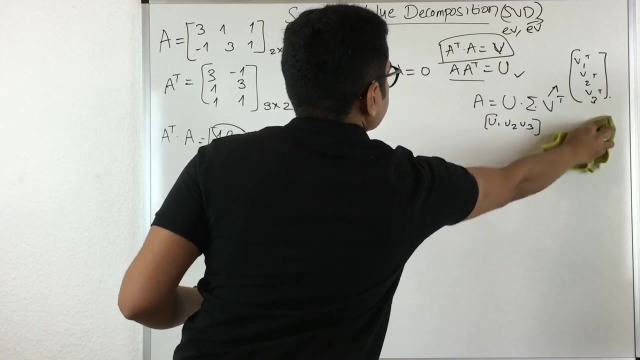 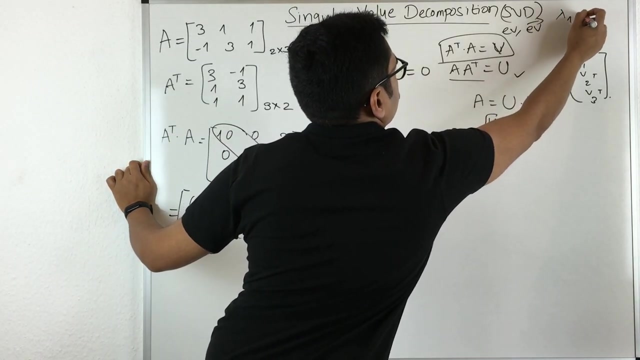 this how we arrive at that. So for the time being, we have to just plug in these values so that we get this V matrix. So now, this step, next step, we would be preparing our V matrix. So how do you prepare that? So now, first we have this value that is: lambda 1 is equal to 12.. I'll just rearrange this. 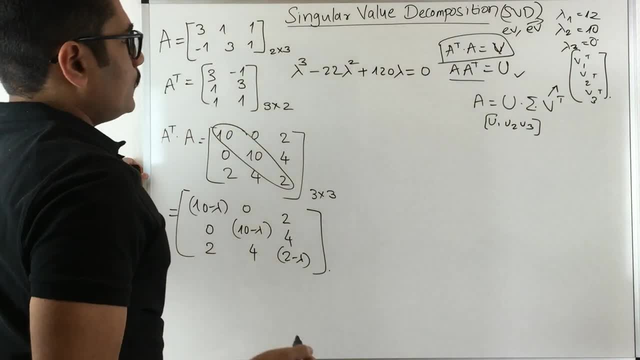 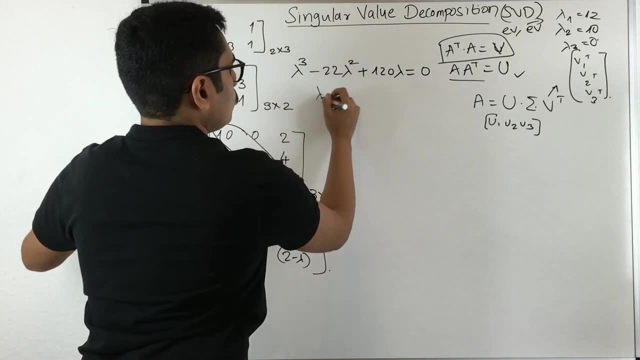 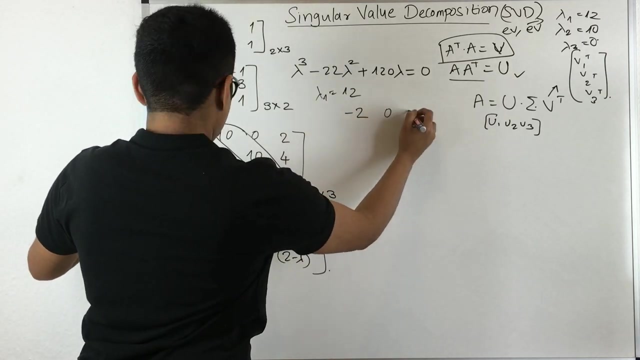 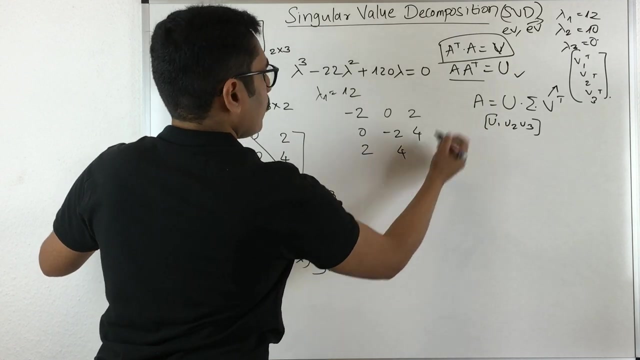 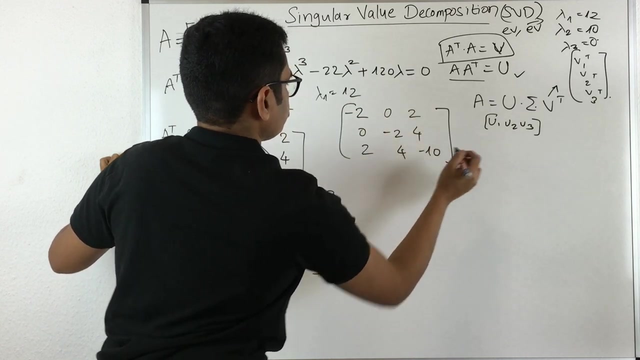 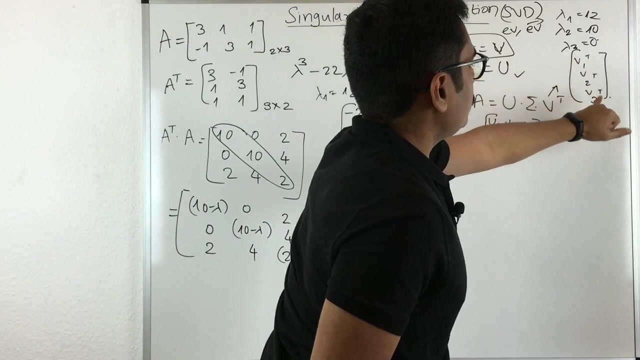 lambda 3 is equal to 0. Now, first, what we need to do is we need to put lambda 12 into this. So when we put a lambda is equal to 12, we get this equation or matrix as minus 2, 0 minus 2, 4, 2, 4, 2 minus 12, that is, minus 10.. Now you need to compute the values of V1, V2. 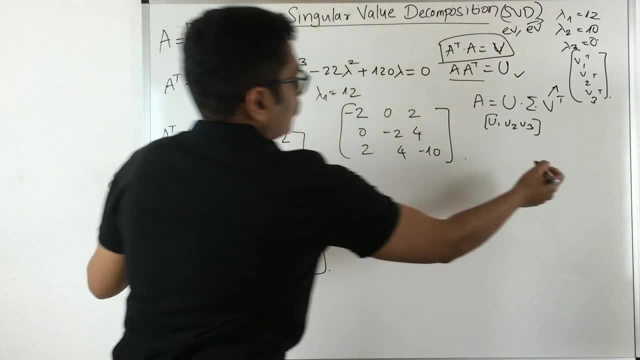 and V3. So this you can just assume. So you have this equation: a minus lambda i x is equal to 0.. Now, for the time being, we have to compute the values of V1 and V3. So this you can just assume. So you have this equation: a minus lambda i x is equal to 0.. Now for the time. 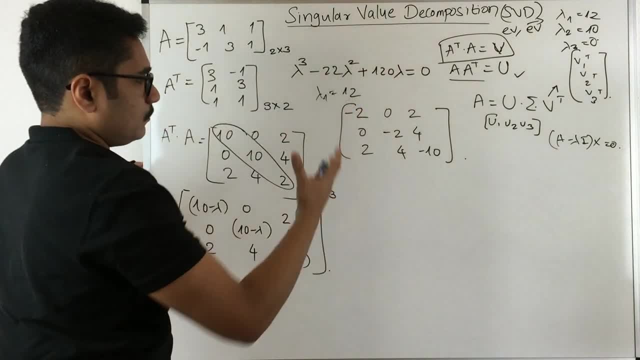 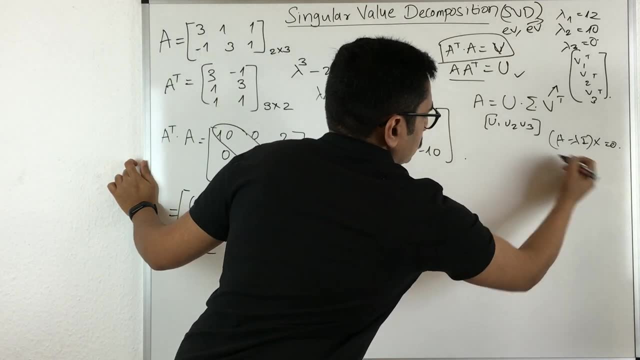 being. we have this equation: a minus lambda i x is equal to 0.. Now, for the time being, you have this equation and you will be in a particular matrix. We are having this characters equations. So for each of these lambda values, we have to calculate this x, 1, x 2, x 3 values. So this can be considered like. you have this X 1. 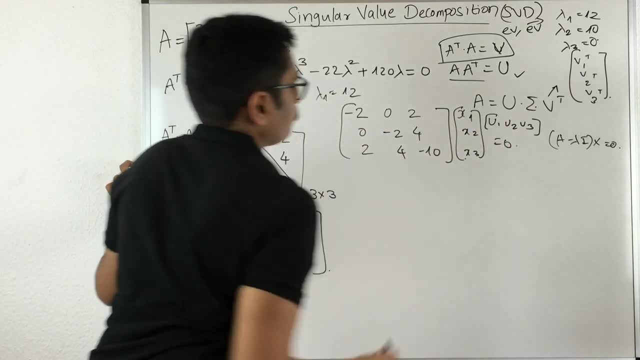 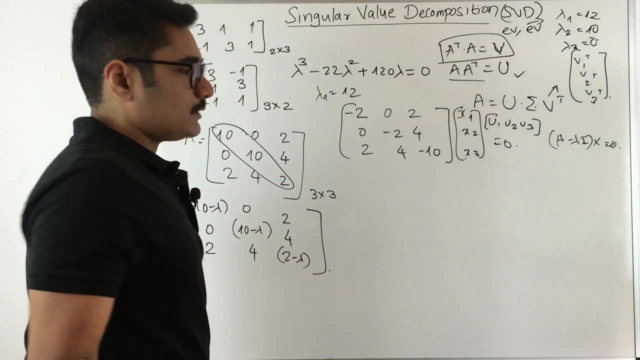 X 2 and X 3, which is equal To 0, now in order to find that we need to apply Kramer's rule. So Kramer's rule is also which is seen in linear algebra. So this is all done in the lower standard. So you 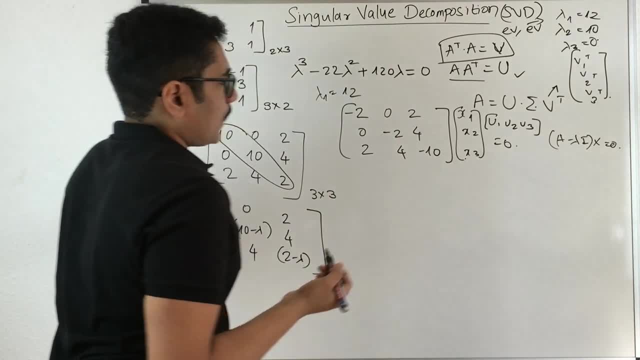 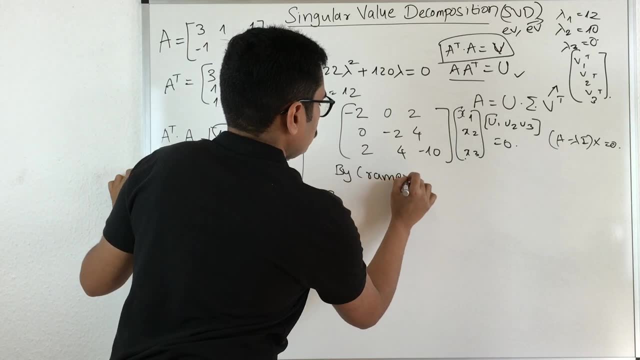 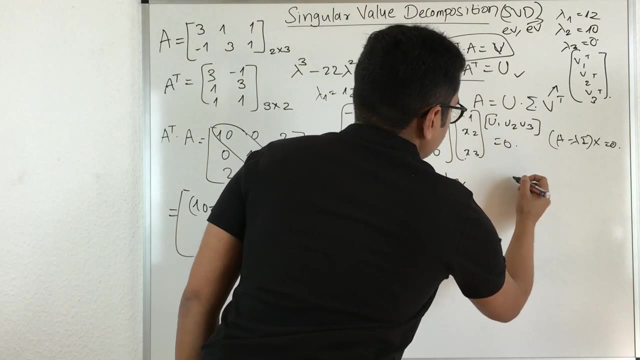 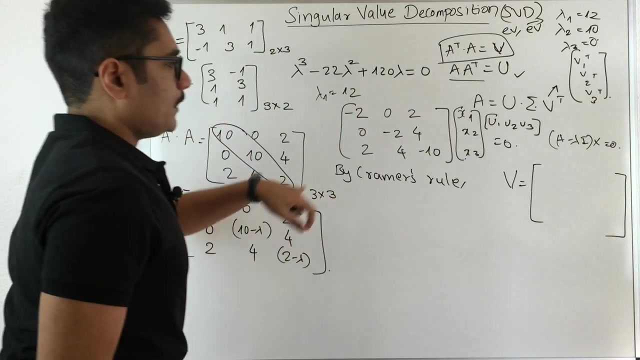 can just have a reference over this. So let us just apply Kramer's rule over this and see how this is computed. So by Kramer's rule we obtain the values for x1, x2, x3.. So where we need to put us, we have to put in our V matrix. So we'll just prepare this by computing all of this. 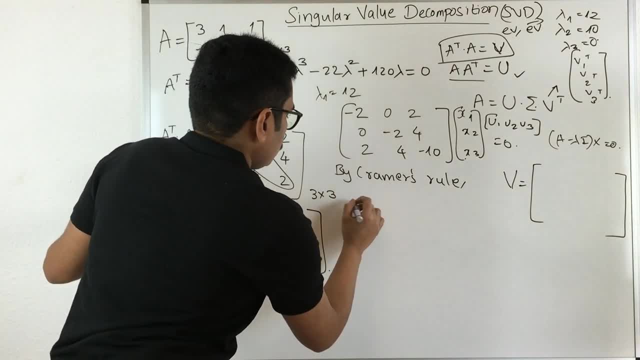 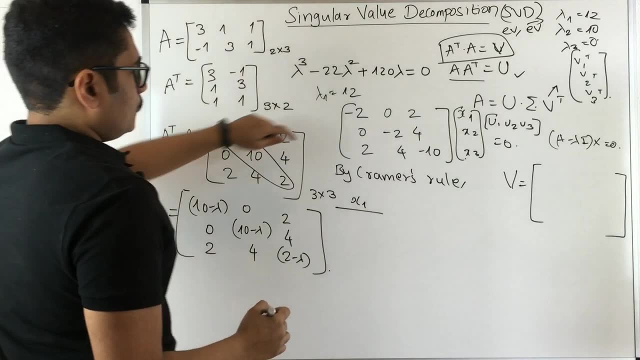 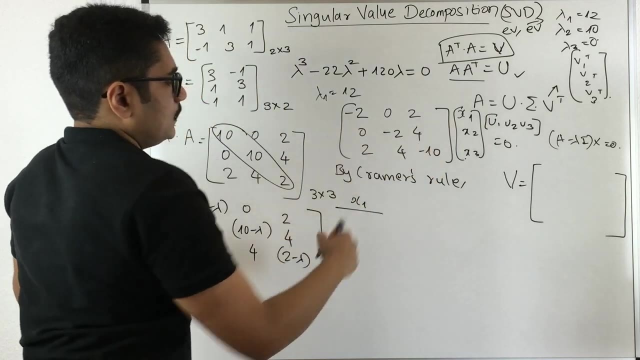 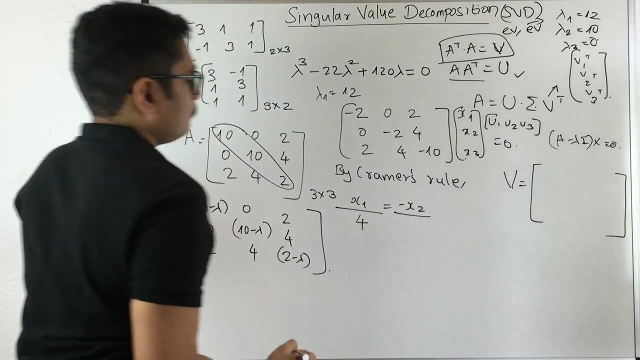 in step-by-step approach. So what we do is we take this x1, so we have x1 upon you. just compute for this. that is this way: that is 20 minus 16, that is 4. then you have a minus x2 here, because that is the second value, and then you have x3 here. So next second value. 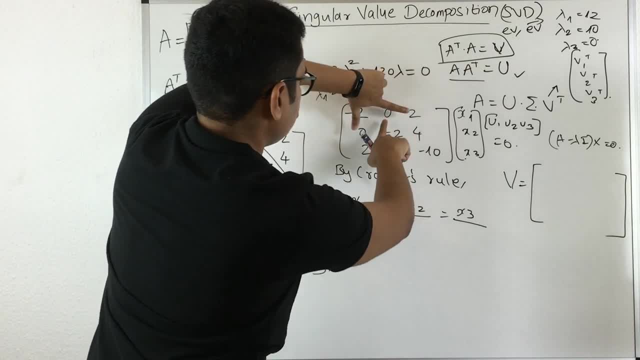 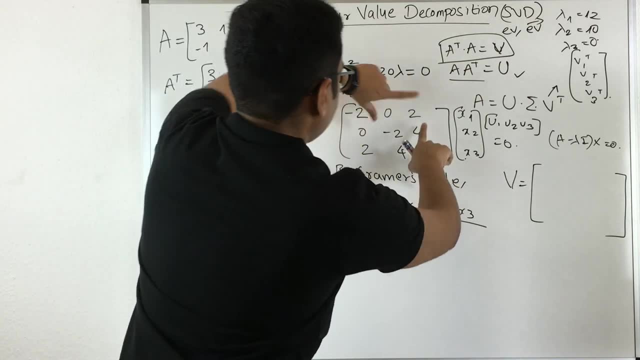 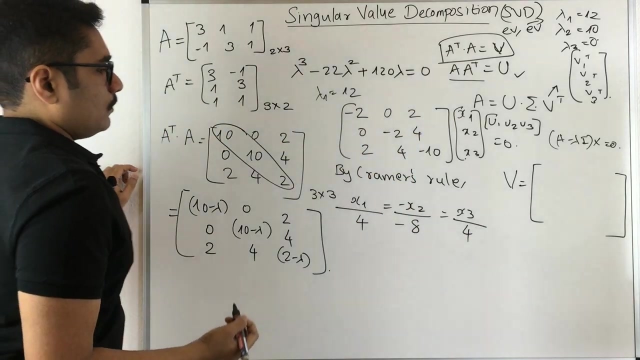 is This. you compute this way, that is, you just consider the 0 here, So that is 0 minus 8, and x3 is this one, So that is 0 minus n minus 4.. So if you just factorize this, so just you. 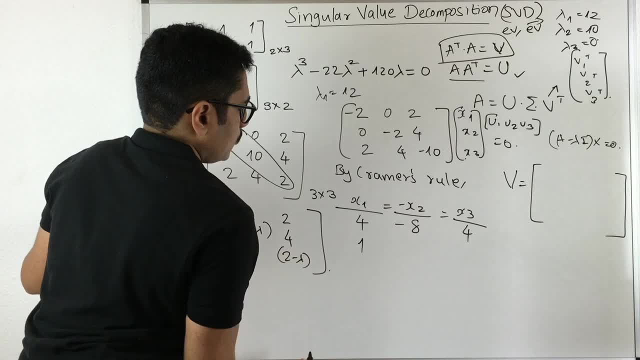 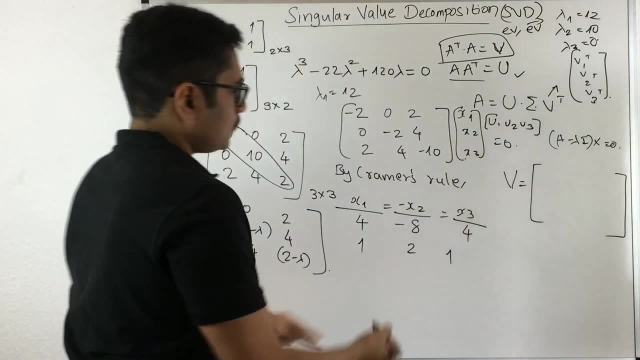 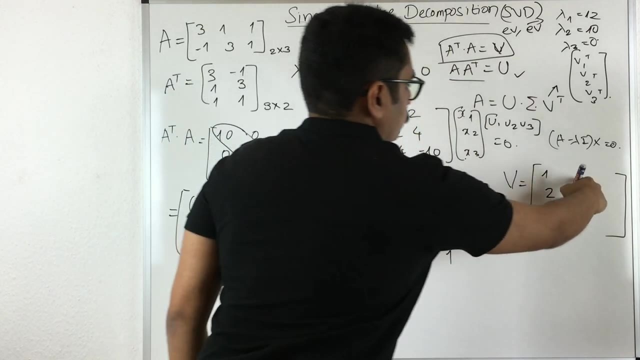 can multiply throughout by 4, you get this as, or divide throughout by 4, 1, 2 and 1.. So now you have to Writing the column view by, because it's a column matrix, so you have to write one, two and one. Now you have to more entries. 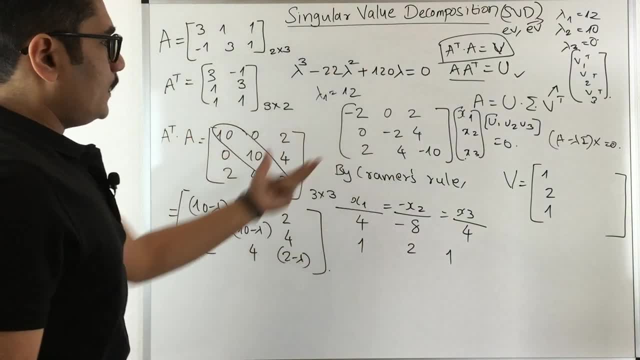 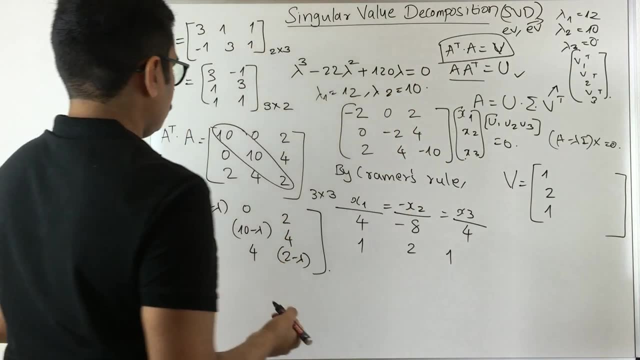 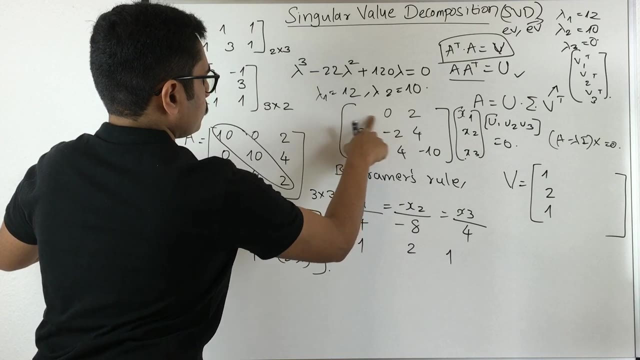 So you'll do in the similar fashion, like how we did for this. So now we take lambda 2 s 10. so how this equation changes. so when we take lambda 2 s 10, so this becomes 0. So this is 0, and similarly here. 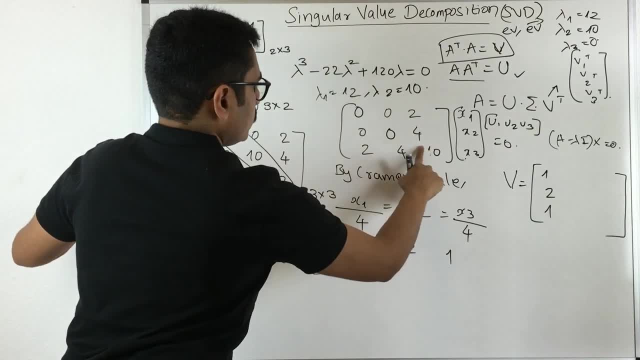 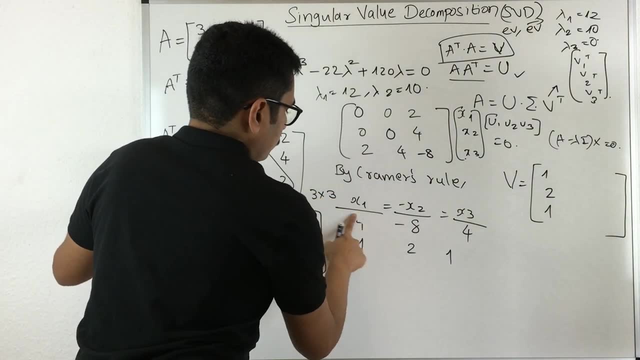 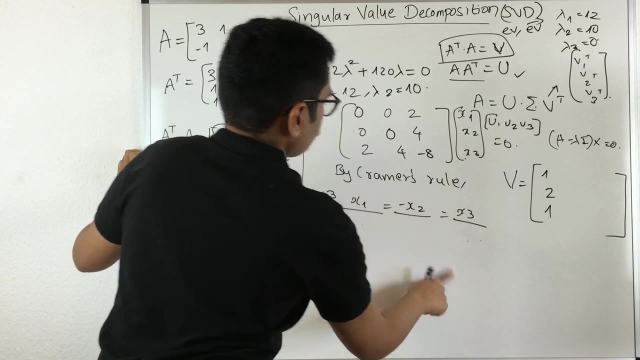 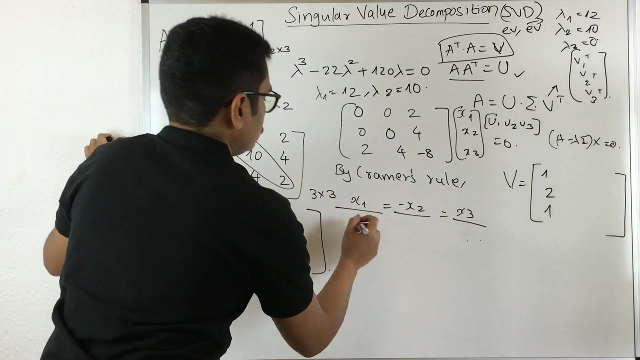 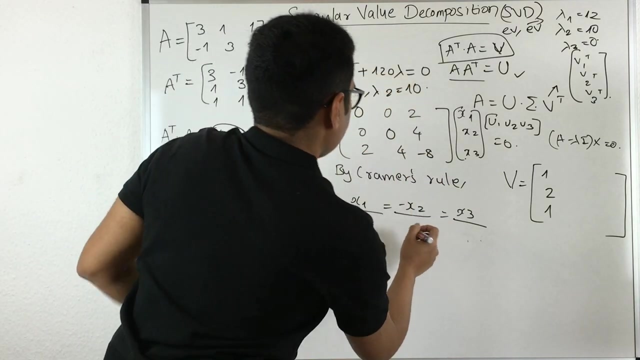 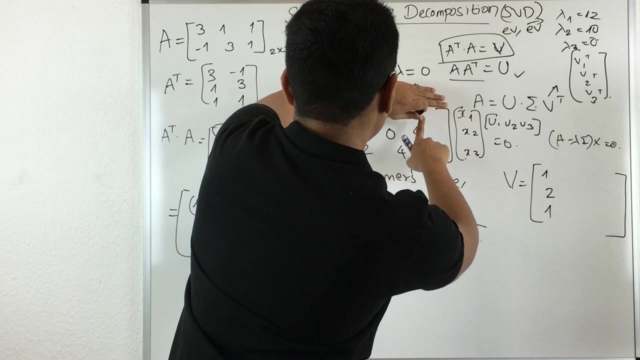 here you have 0, and this is 2 minus 10, that is minus 8. now, similarly, by using the Kramer's rule, you have to change this values. So how do you do it? So, in the similar way, this: that is 0 minus 16, then you have 0 minus 8, and then finally you have x3. so that is this value. 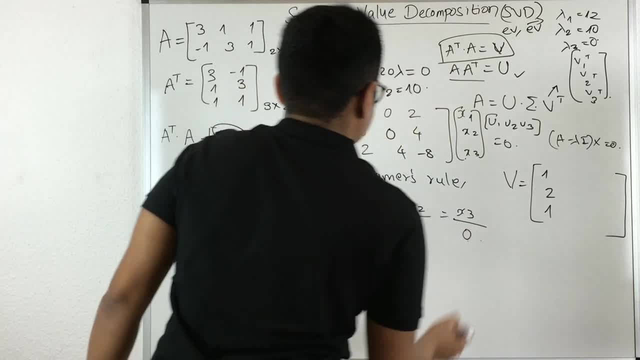 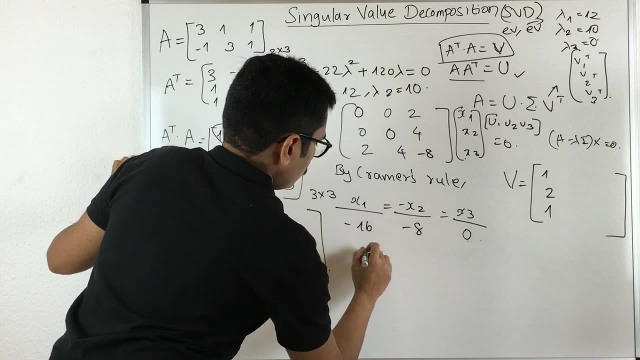 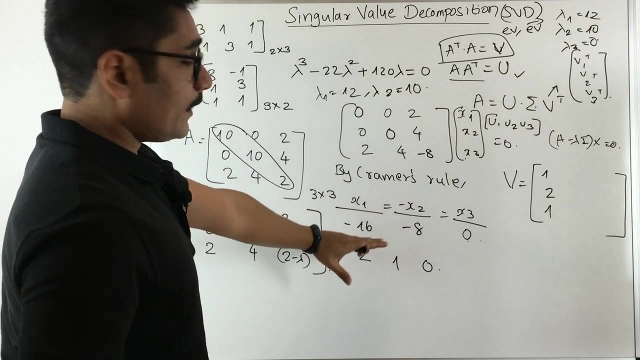 0 minus 0, so that is 0 itself. So when you just divide, so you have this 2, 1 and 0.. Just I'm just multiplying by or dividing by minus 2 so that I get as this entry. So now, 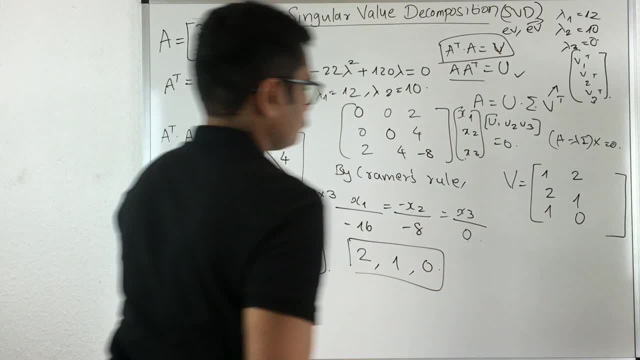 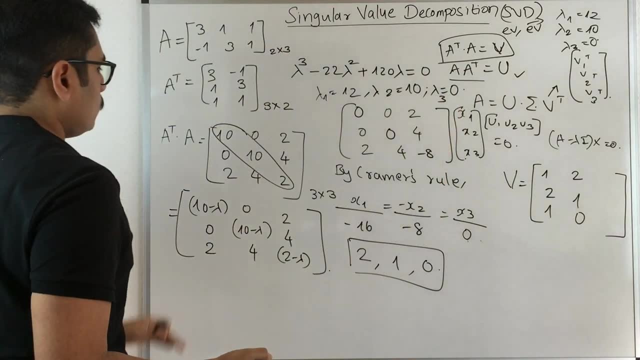 this becomes our column 2, 1 and 0. now, similarly, when we put lambda is equal to 0 or lambda 3 is equal to 0, we get this equation back. that is our normal one. So we have 10 0, 2. 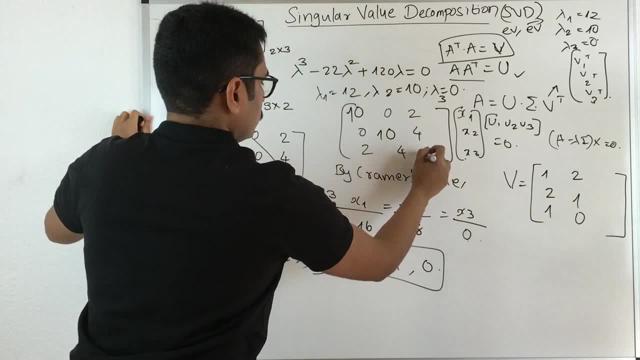 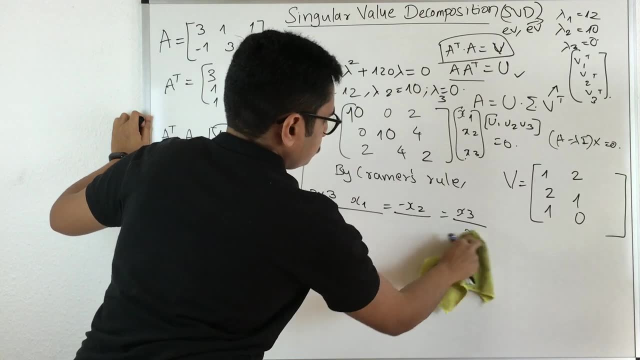 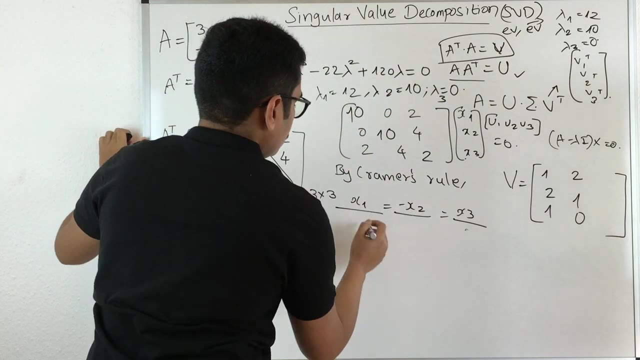 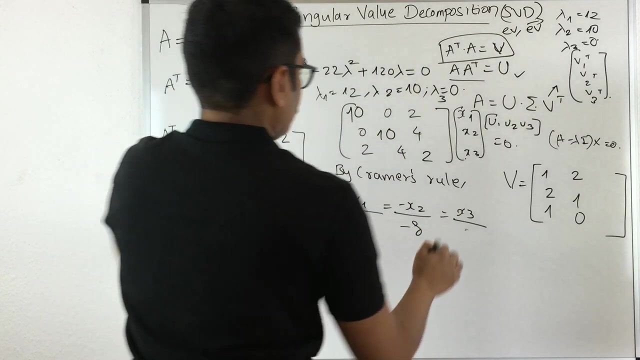 0, 10, 4, 2, 4, and here we have 2. so similarly we change this equation. What we obtain is: we have 20 minus 16, that is 4, then we have 0 minus 8.. Then we have 0 minus 20.. 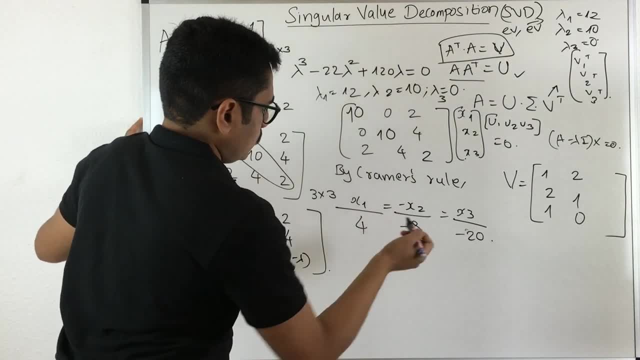 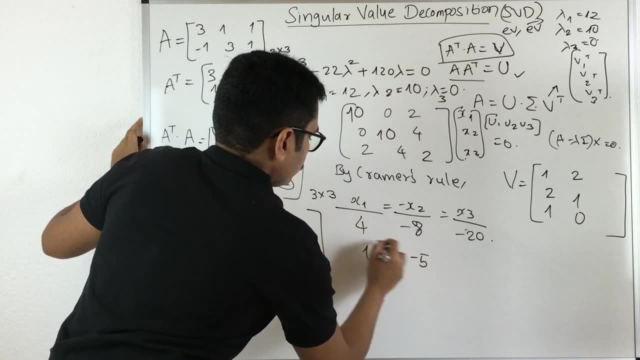 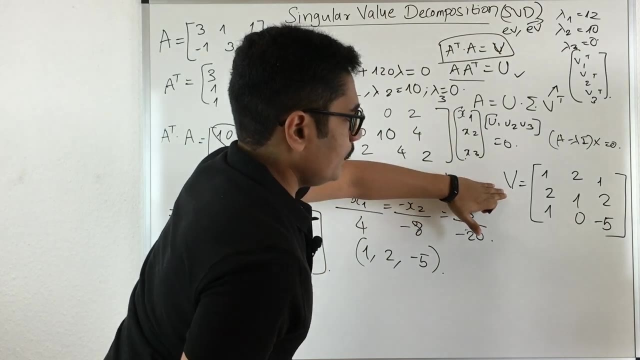 So we just divide throughout by 4. yes, for so we get four. ones are then 4, twos are and 4 minus 5. so you write this in column 1: 2 and minus 5. now this is our V matrix. but 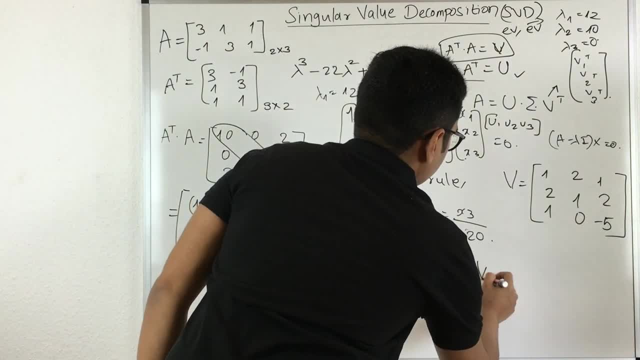 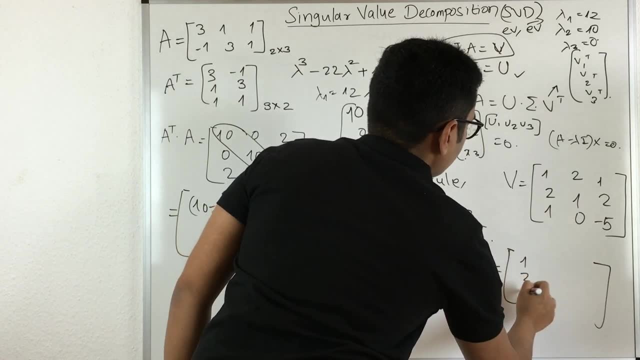 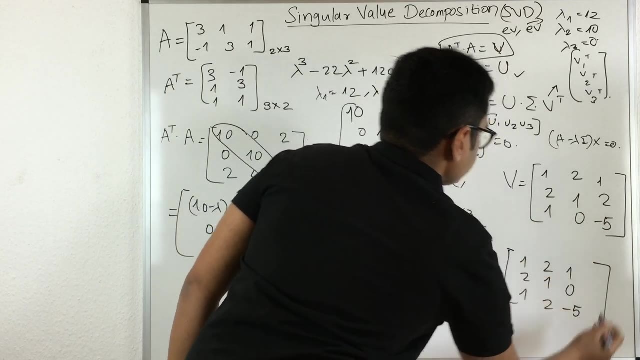 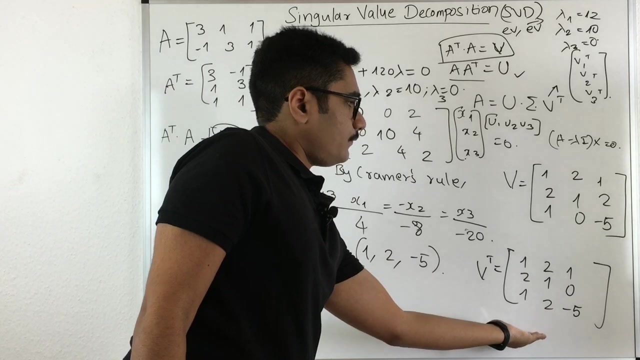 we want V transpose here so that simple, just convert the rows into columns, So this: 1, 2, 1.. 1, 1, 1 and remain the same. then you have two one and two, then this one zero and minus five. Now this, what you see, is this is just the matrix that we have obtained from all of this. 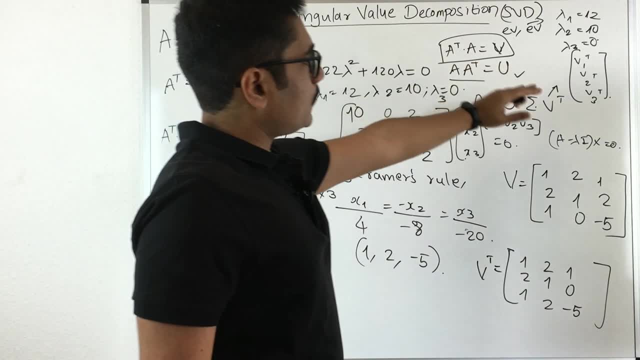 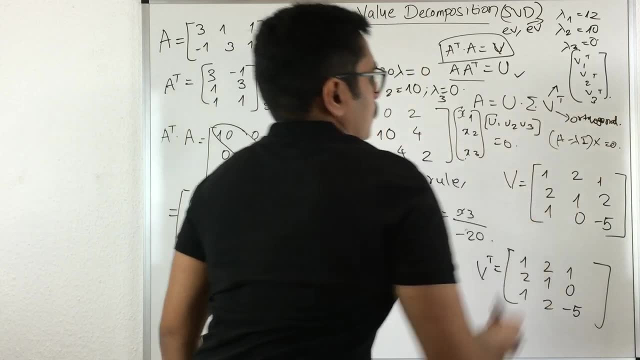 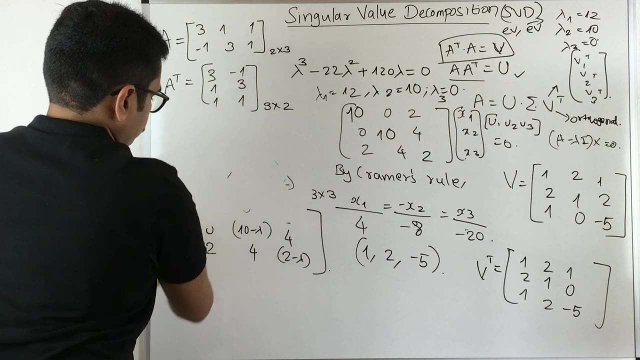 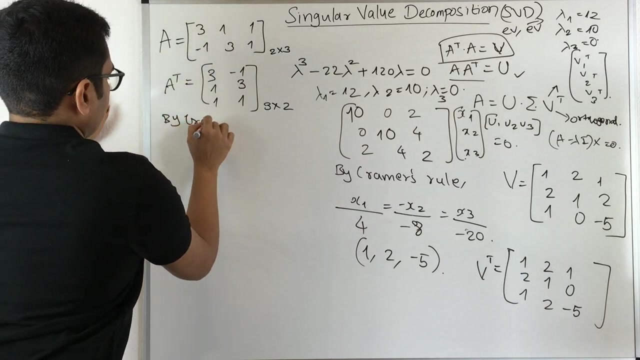 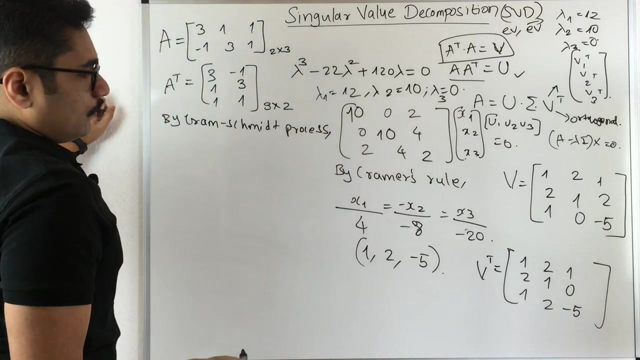 process. But what SVD says is that this particular last Matrix is also an orthogonal Matrix. So by the Gram Schmidt process you do the organization. So by Gram Schmidt process Of orthogonalization, what you do is you calculate the length of this along the rose. So you 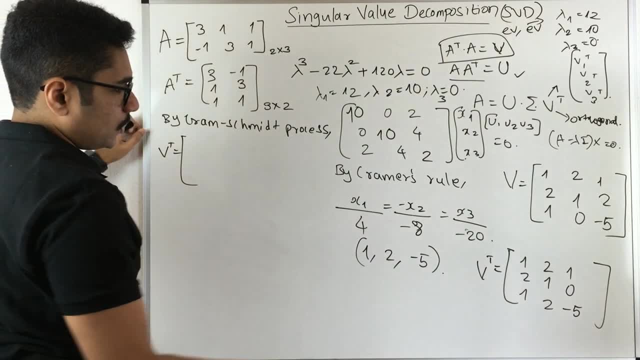 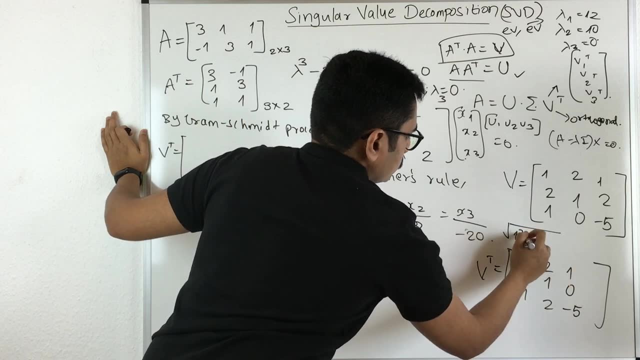 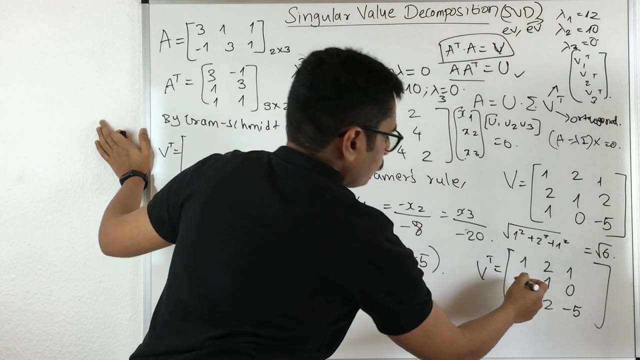 have this v transpose as after applying the organization, that is, if you just consider the length. so that is square root of sum of squares. that is 1 square plus 2 square plus 1 square, you get it as root 6. similarly, for this you have: 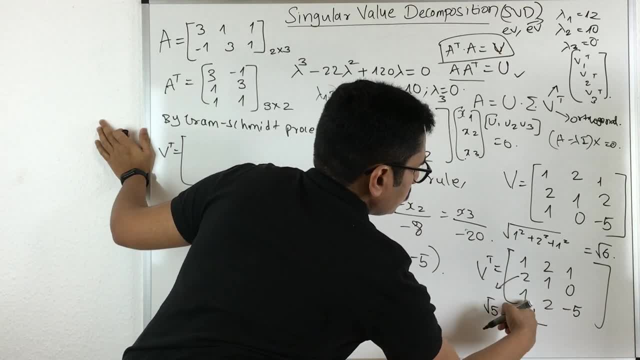 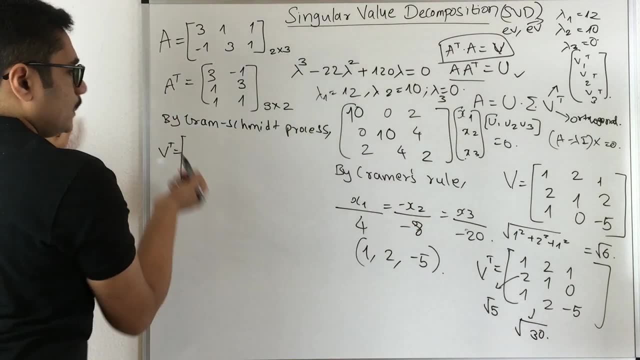 root 5. similarly, for this you have, that is, 1 square, 2 square and 5 square. that is, you have root 30. So you just have to divide this, so that is 1 by root 6, then 2 by root 6: 1. 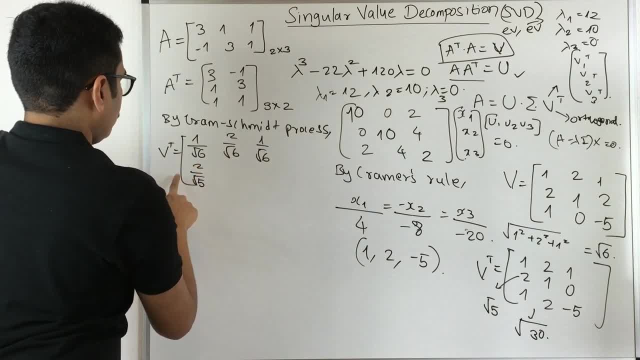 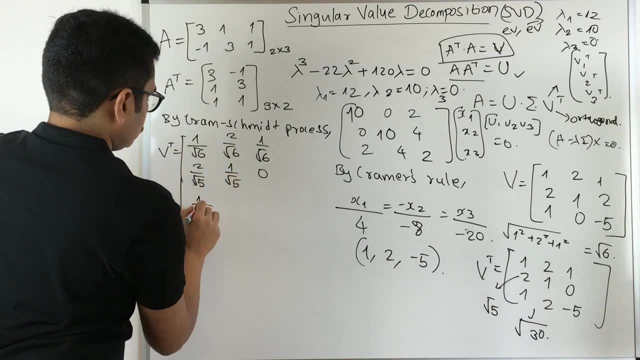 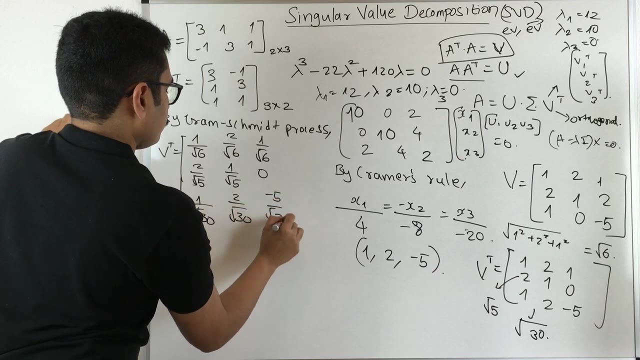 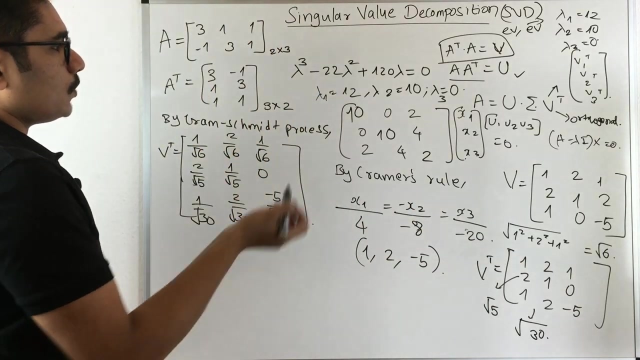 by root 6, 2 by root 5, 1 by root 5. that is 0. this is 1 by root 32 by root 30 and minus 5 by root 30. So this is our final matrix. what we get now are last and final job is to obtain are diagonal matrix which. 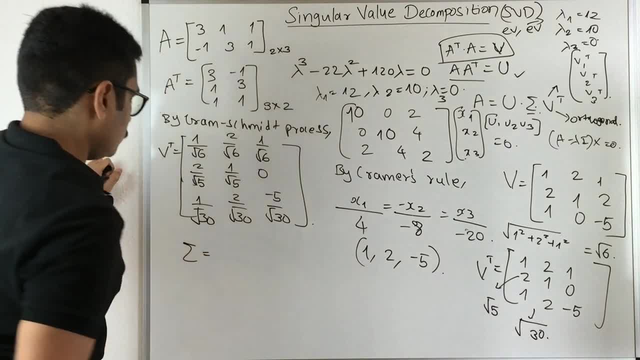 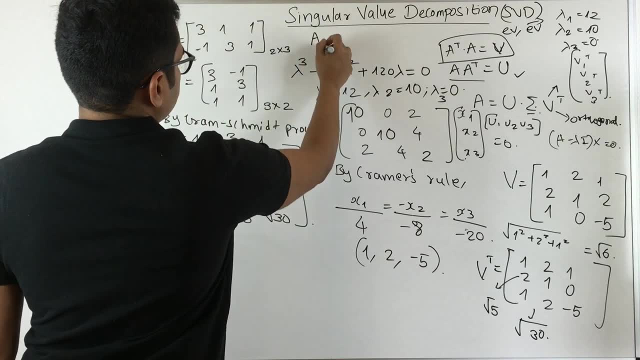 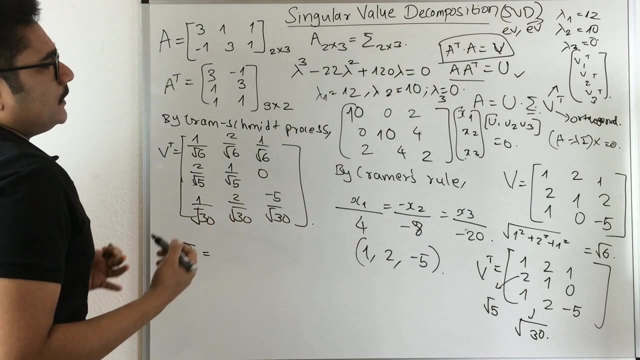 is of singular values. So how do we obtain Sigma? So Sigma, if you see from the basic definitions, So that is of the same size as your a. so if a was 2 cross 3, then your Sigma would be also of dimension 2 cross 3. now what will be the values of this? So if you just 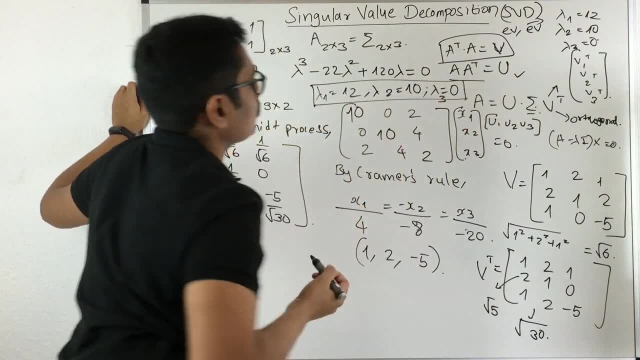 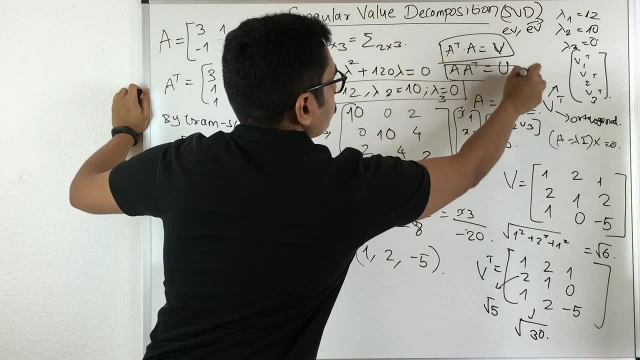 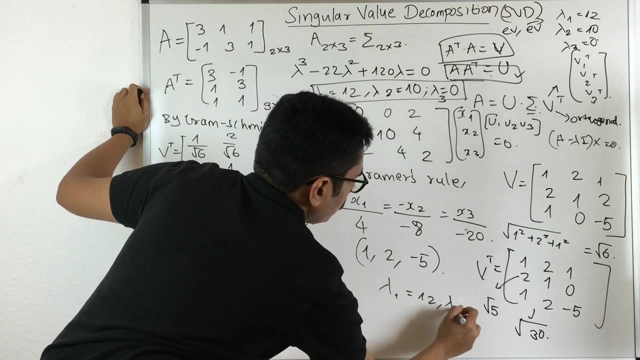 look at this: Value values, that is, eigenvalues, and if you just see the values which you obtained from this as well, So with a transpose for you also, you got the values, as Lambda is equal to 12 and Lambda is equal to 10.. So you can see that there are two values which are repeating. 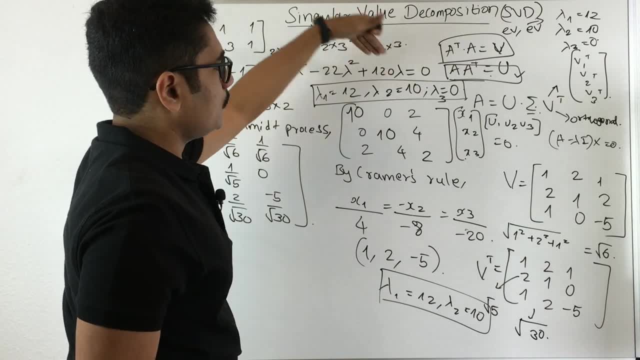 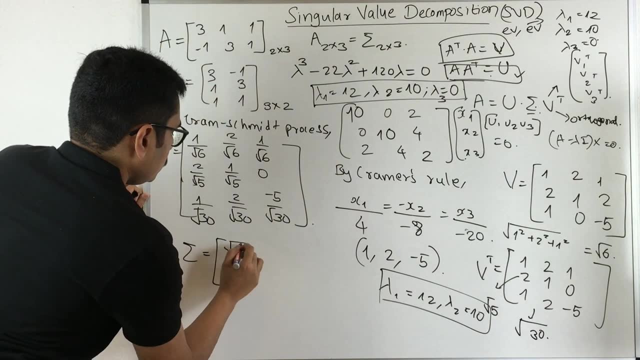 that is 12 and 10.. So essentially these two are the unique values which you obtained from that singular matrix. So how do we write this? we just write the higher value or the higher eigenvalue up here. then you have to zero values here: 0, root, 10 and. 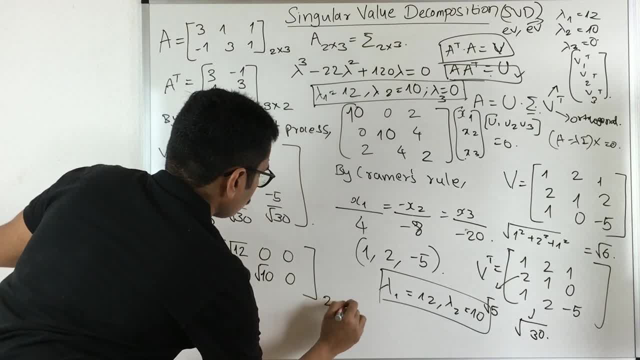 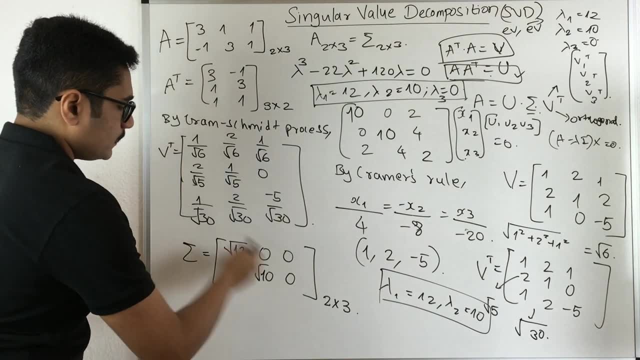 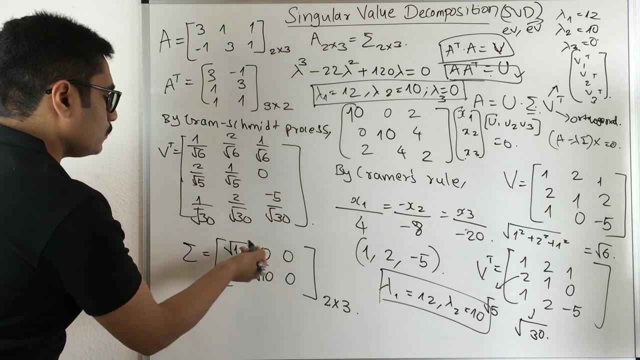 0, so which is also at 2 row and 3 matrix, 3 column, sausage matrix. now Why do we write this? why? because it's written. that is singular. There is written in an increasing localizing way, So root 12 has higher value. So say, for example: this value comes out to be square root of 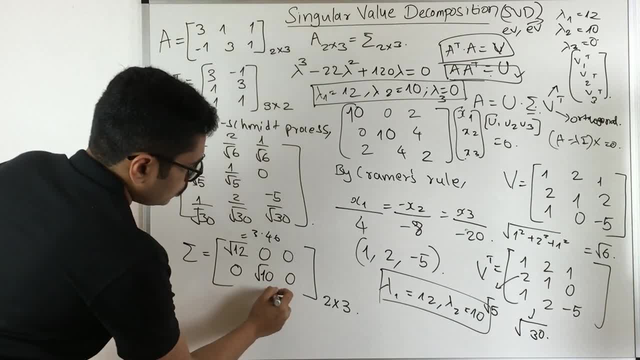 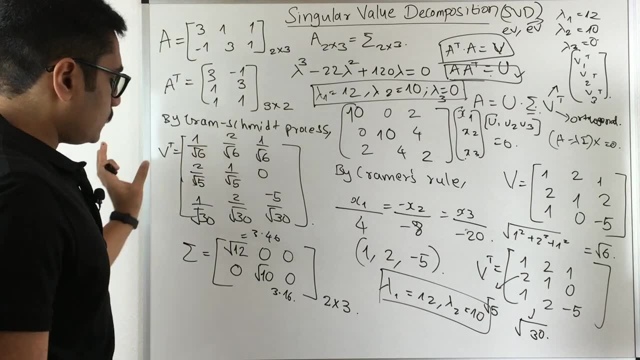 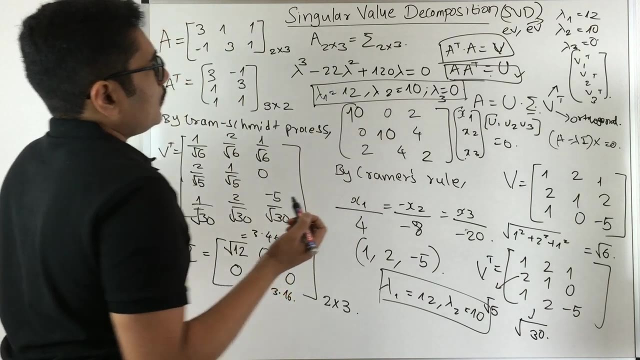 12 is 3.46 and square root of 10 comes out to be 3.16.. So you have to write this matrix in such a way that the higher value comes, or the higher square root value comes first and then the lower one. Now this is how we solve the singular value decomposition. but 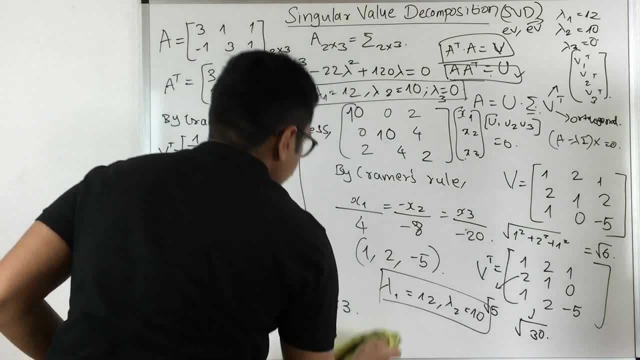 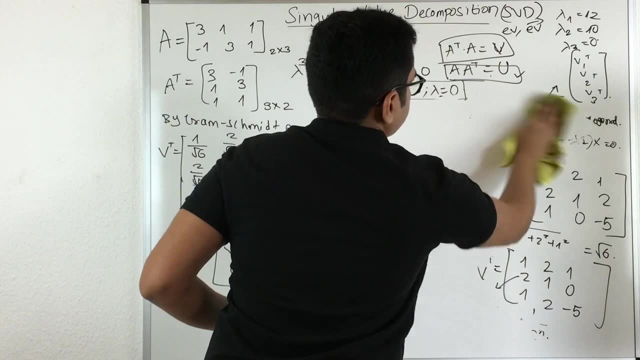 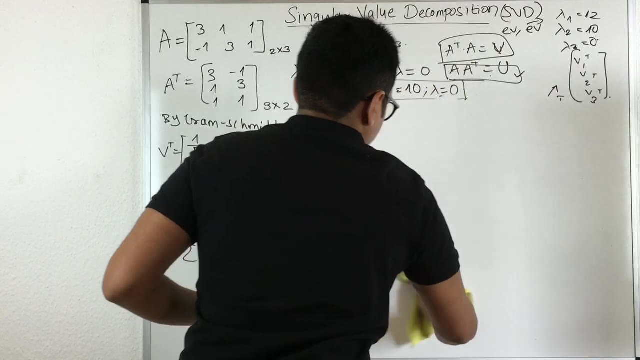 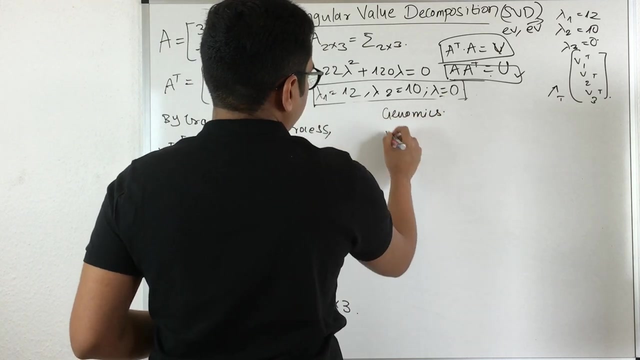 in real world You have many applications of singular values. So when we talk about genomics, There we mainly use the singular values. So where you have certain gene samples, so in Genomics, so certain people's are there and save, you have person, a Türkiye. 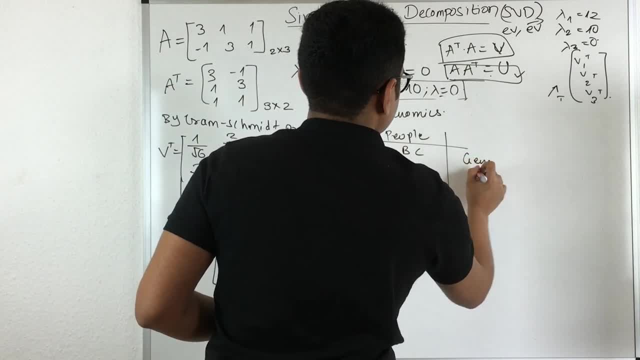 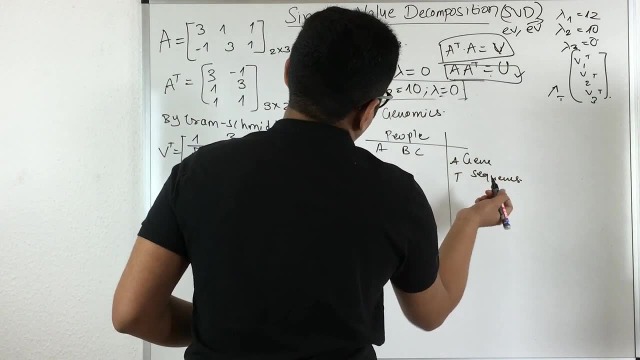 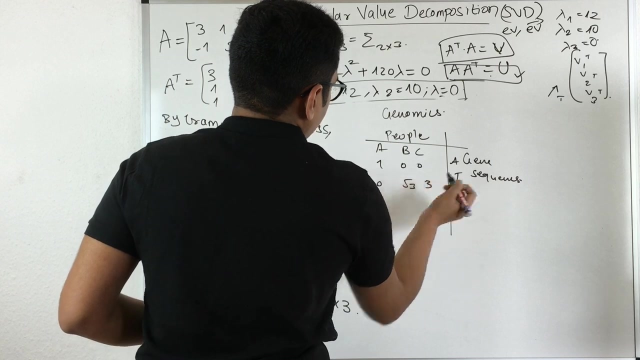 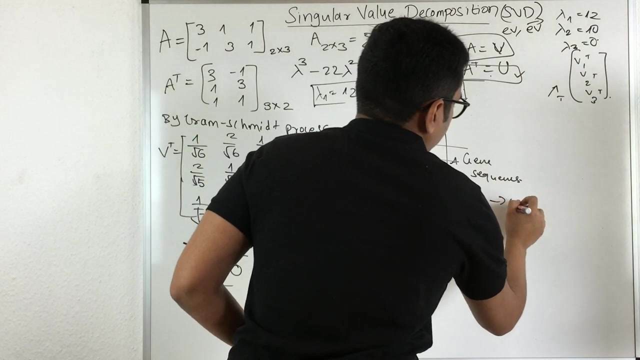 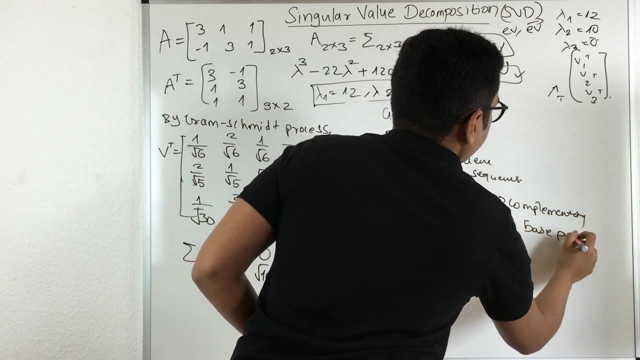 be C. then you have the gene sequences, Say you have the ATGC strands, that is, adenine, thymine, then guanine, cytosine. So you have some entries and some values here, like three something, something values. So this is essentially used for the complementary base pairing. Now 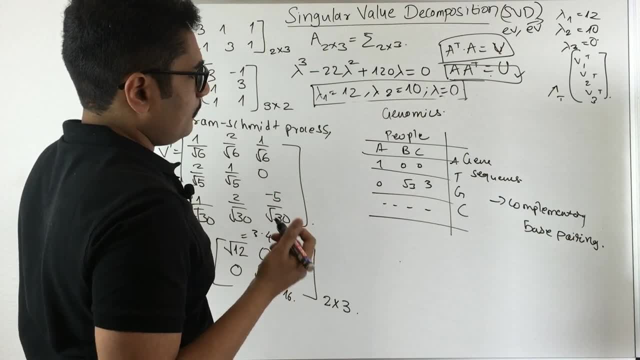 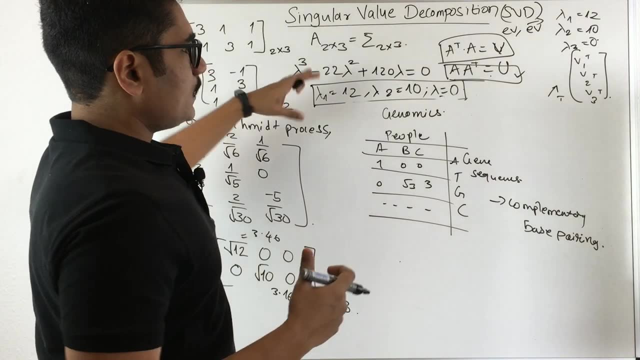 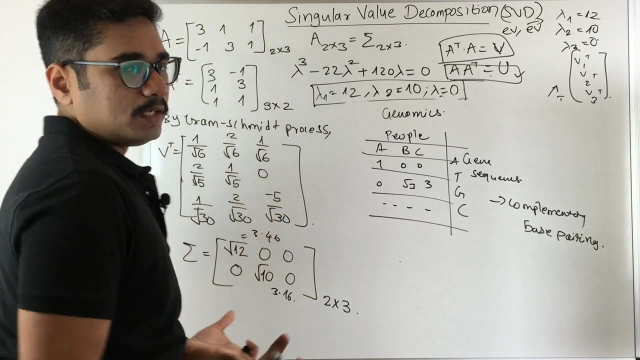 this is done in order to check if some particular people suffers any gene disease or gene level disease in their DNA sequences. So here in this example, we have just limited our dimension just for Right Right representation purpose, to only this much. but in the real world you will have a huge. 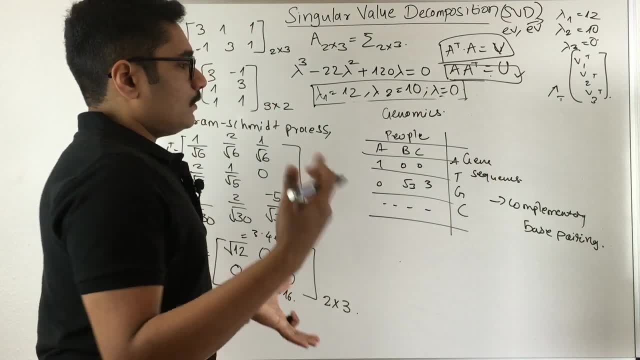 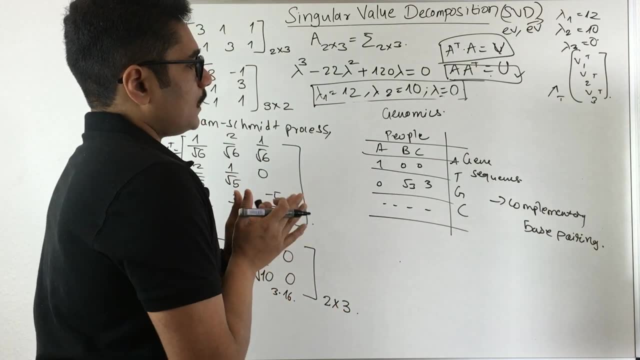 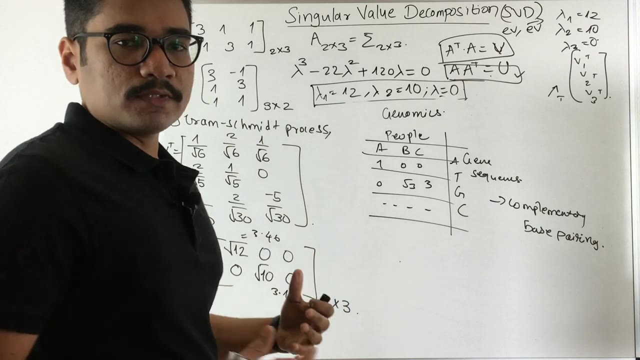 number of matrix. So, say, you are doing a drug test. So, like the recent times, you have this coronavirus breakdown. So what you have is we have a large pool of people who are suffering from this. So we have to see the gene sequences of each of them and we have to test whether 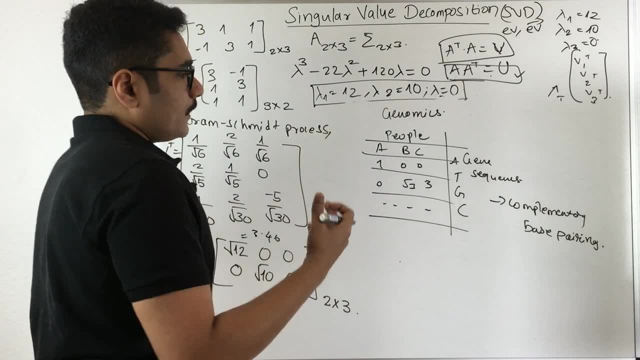 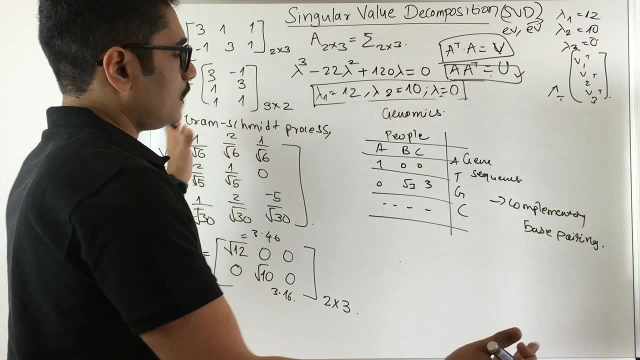 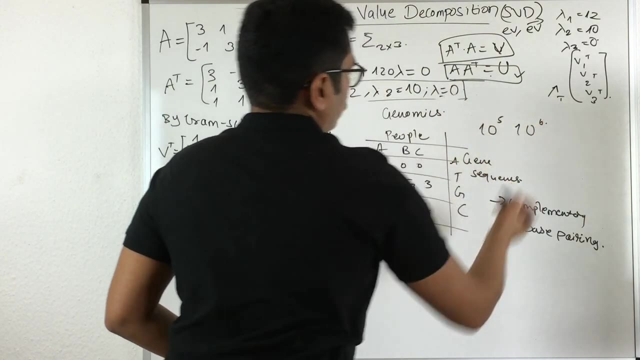 they are really a victim or not. So there the role of statisticians becomes very much crucial. So there we mainly use this decomposition. So you can just consider the dimension would be of any size, So it can be of 10 raise to 5, or 10 raise to 6.. 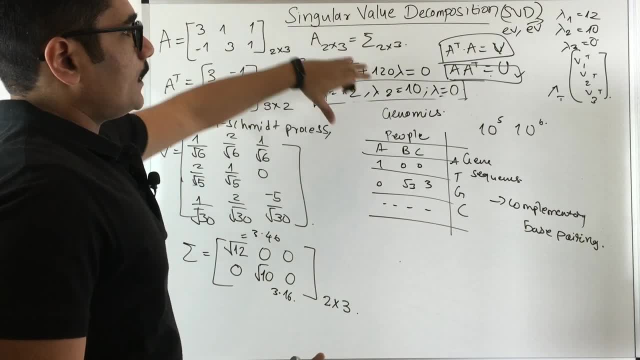 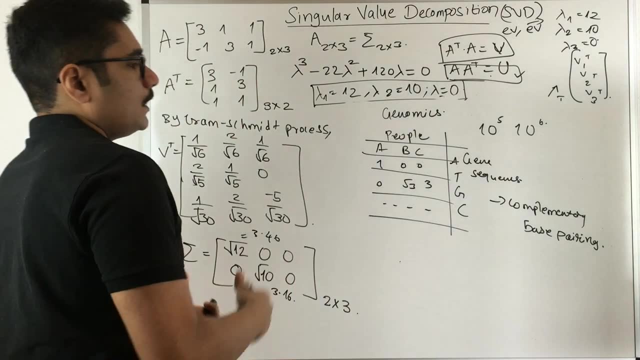 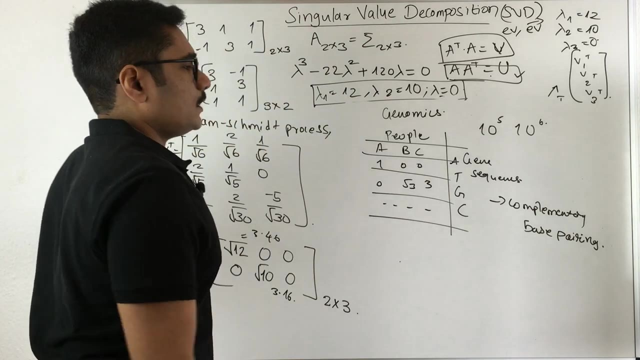 So there, if we don't just reduce the dimension to lower dimension, then it becomes a very complicated activity to do all of this purposes, but you just constraint that limit up to certain level. and to talk about the next application We mainly use in recommender systems: